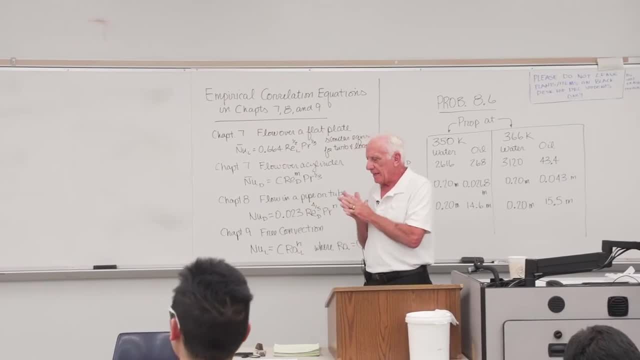 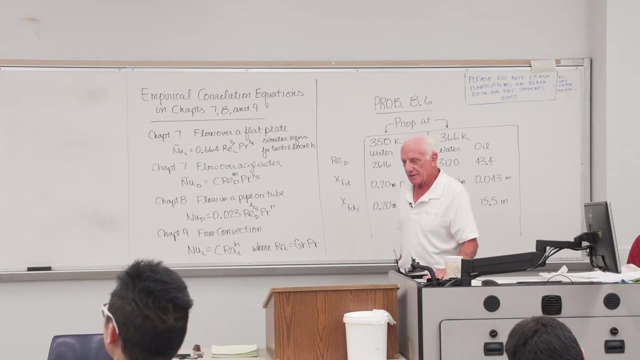 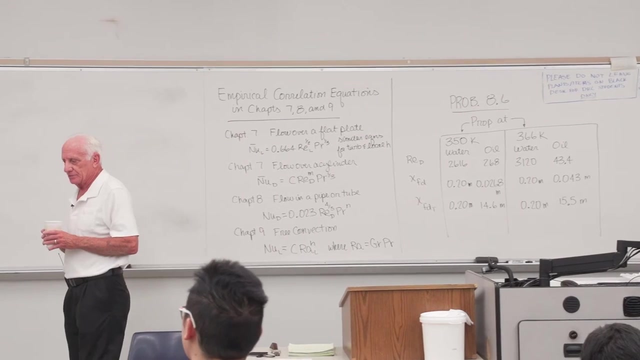 of the two. But let's go back and we've spent the last several weeks on convection heat transfer. We started out in chapter 6, more of an overview type chapter. We got into chapter 7, flow over external surfaces. Chapter 8, flow inside cylinders or tubes or pipes. Chapter 9,. 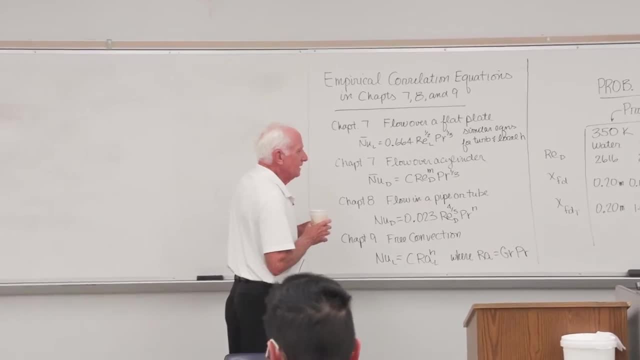 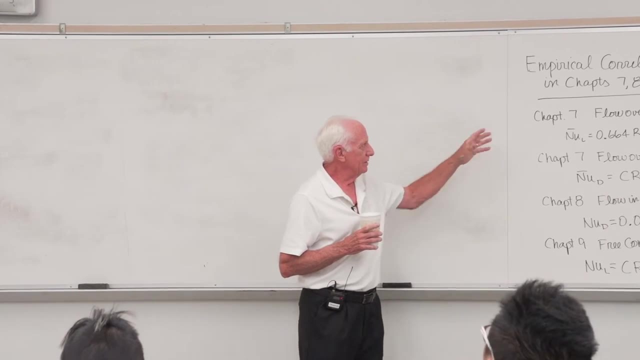 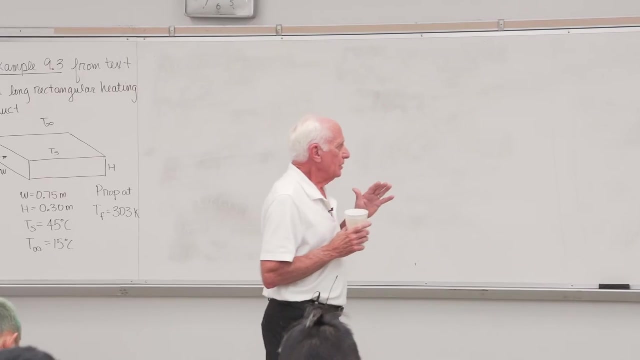 free convection Heat transfer. And if you go back, just so you can see the similarity of these chapters, if you go back and look at chapter 7, now we're trying to find H, because once we find H we can find Q. So 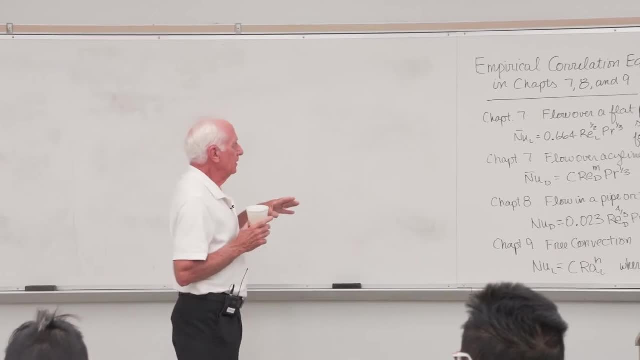 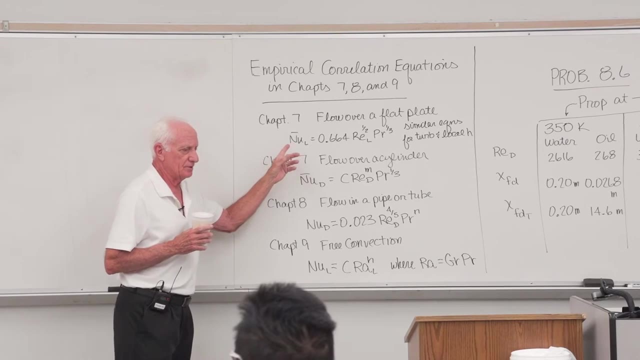 the Nusselt, of course, has H built into it. So in chapter 7, flow over a flat plate. This is just one equation. There are several in that chapter, but I just put it in here. So in chapter 7, flow. 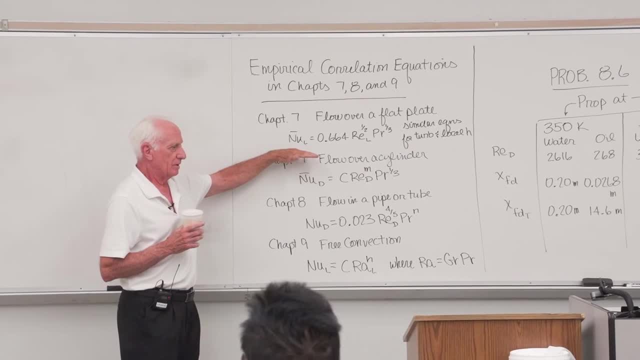 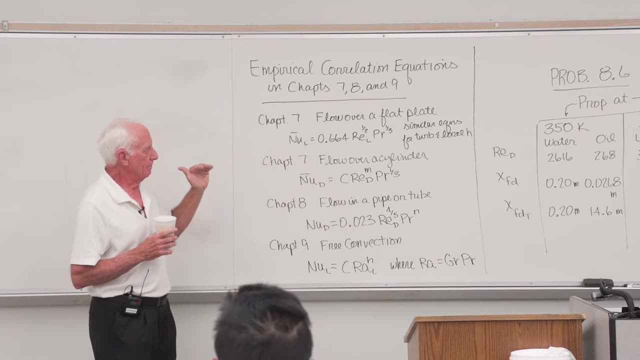 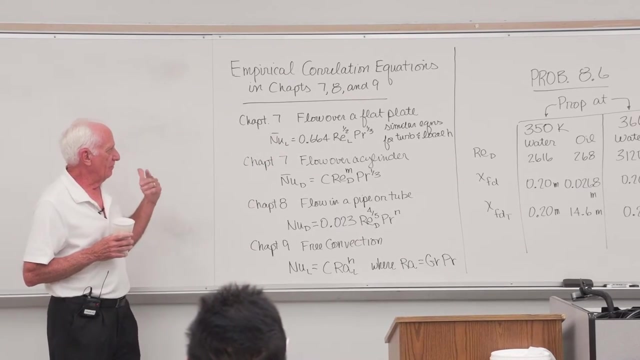 over a flat plate. This is just one equation. There are several in that chapter, but I just put it one down to show you its form. There's different equations for turbulent flow, for local H- This is for average H- But they are very similar to this equation. The last part of chapter 7, flow over a. 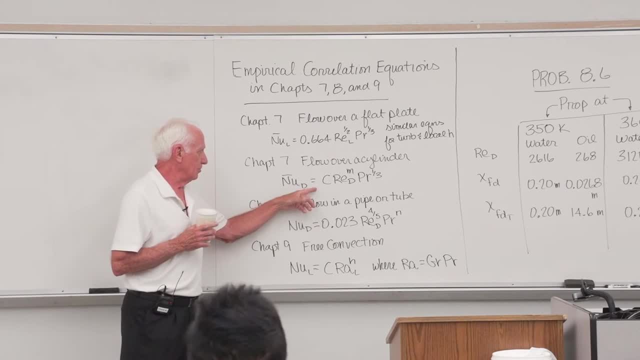 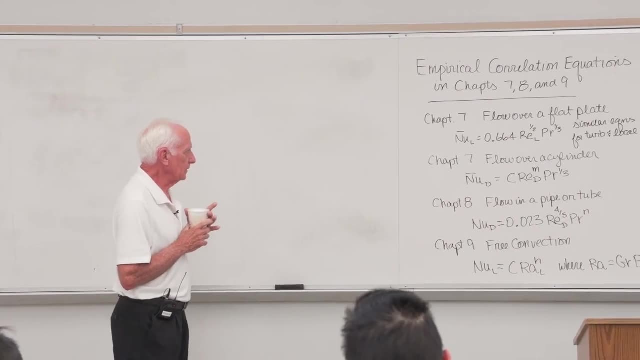 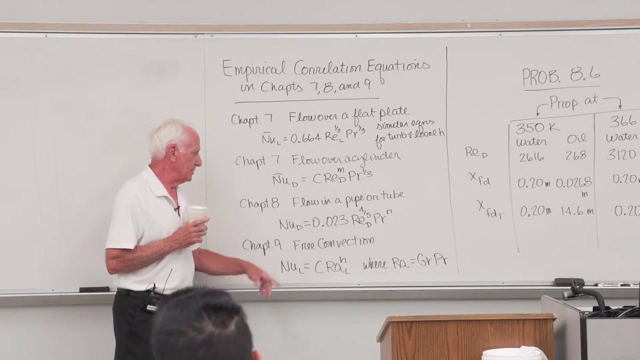 cylinder on the outside of a pipe or a tube. Here's the correlation equation where the constants C and M come from a table. Chapter 8, flow in a pipe or a tube. Here's the correlation equation And it can depend on you know. 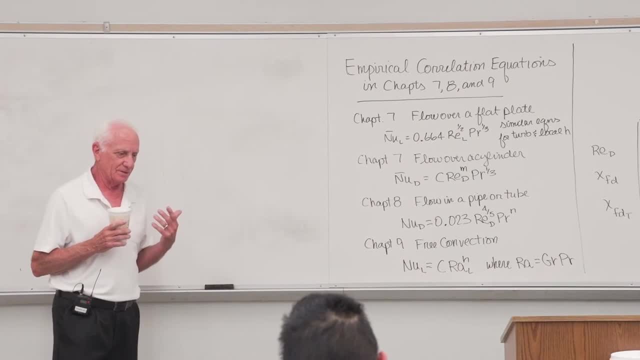 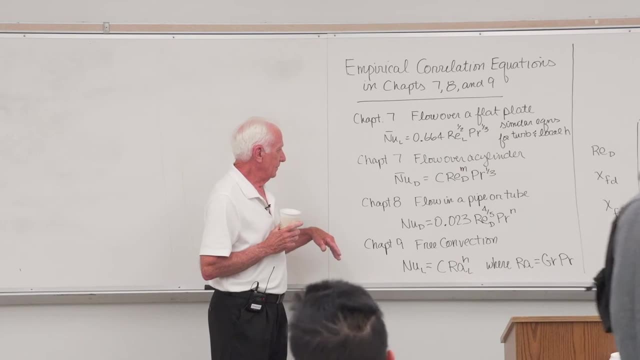 is it laminar, is it turbulent? is it constant wall heat flux? is it constant surface temperature? But anyway, the form of the equation basically looks like this. Now, chapter 9, free convection. here's the form of the equation. 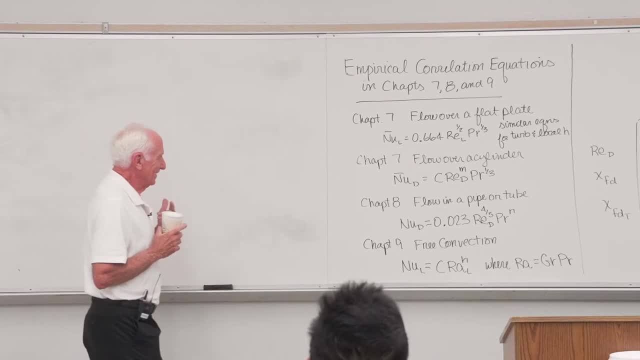 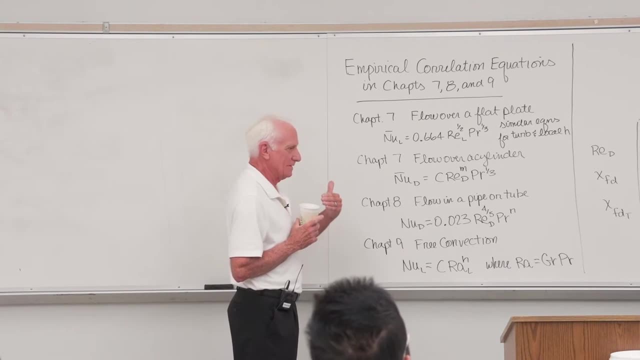 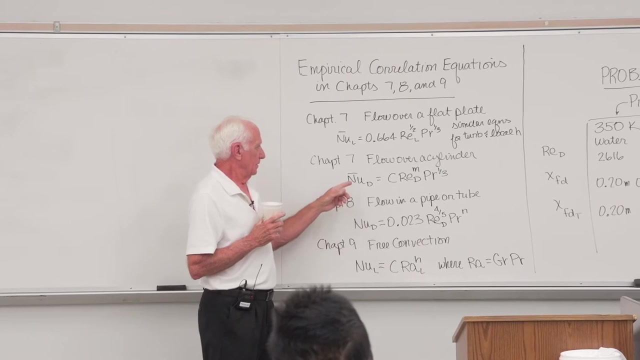 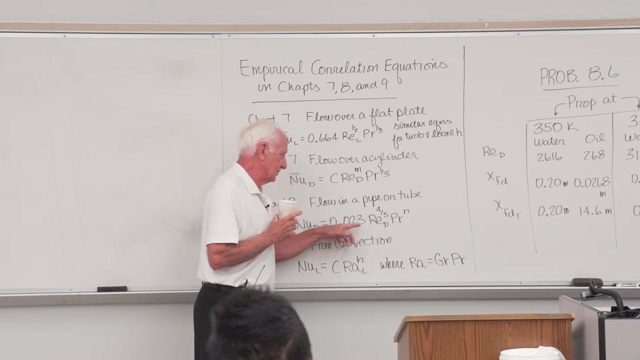 Now look at how similar they are In all these guys right here. the way they correlate the experimental data is by this power law: No salt is a constant Reynolds to a power. No salt equals a constant Reynolds to a power. Chapter 8, no salt equals a constant Reynolds to a power. Chapter 9, no salt. 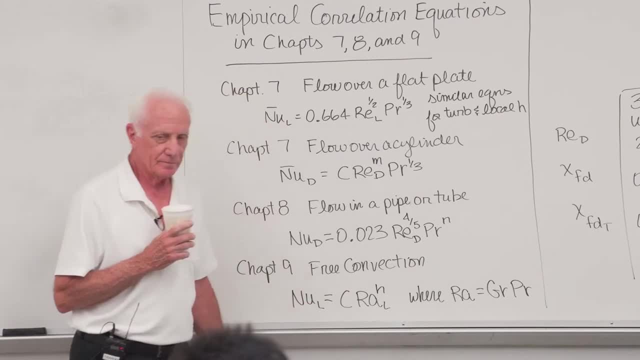 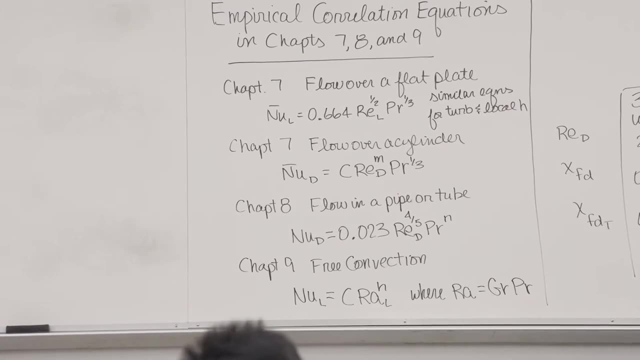 equal a constant Rayleigh to a power. Of course, one of the major differences- chapter seven and eight, it's Reynolds number. Chapter nine: forget Reynolds number. now it's the Rayleigh number, But the form of the equations is very similar. 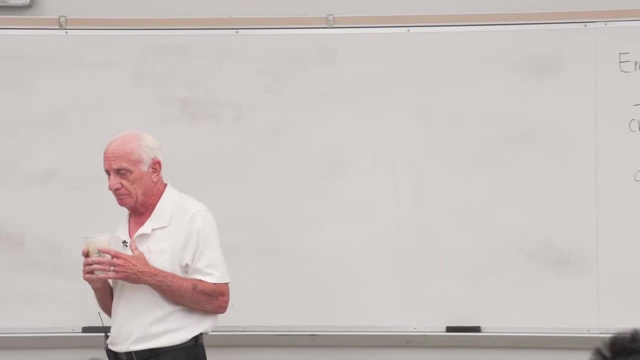 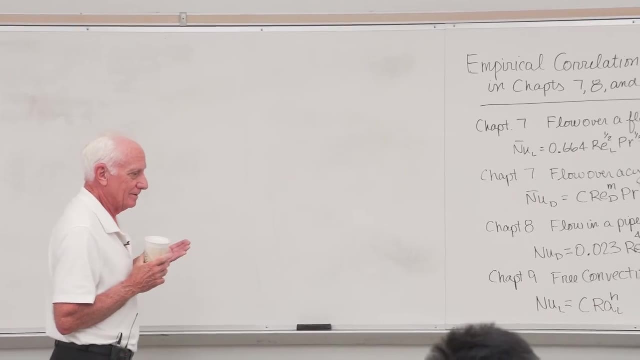 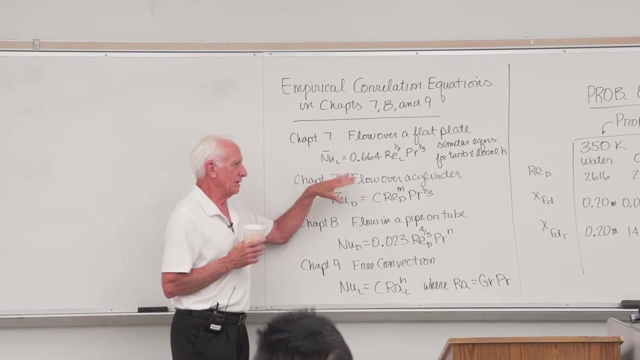 We engineers love that kind of correlation. It's a power law correlation. So you can see the similarity in three chapters of convection heat transfer. Most of the basic correlation equations are Nusselt, equal, a constant, Reynolds or Rayleigh raised to a power. that's it. 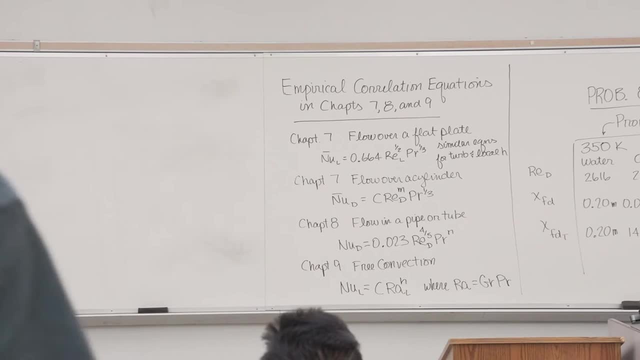 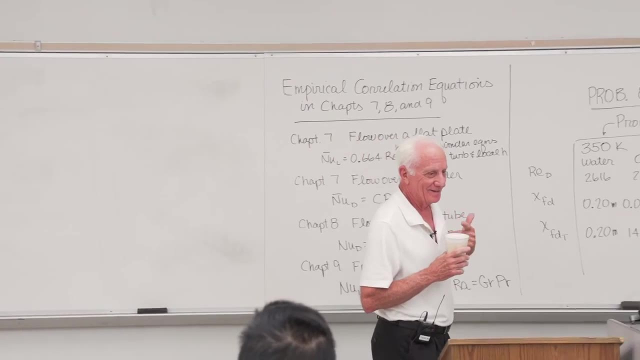 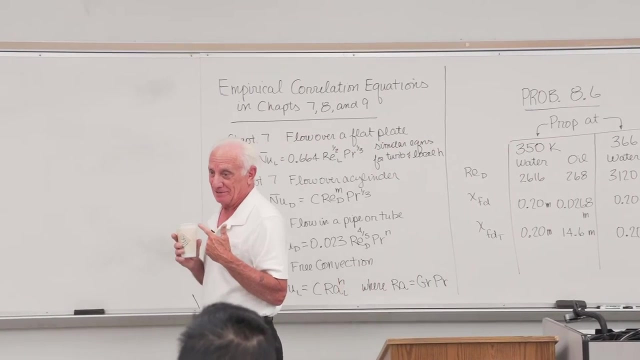 There's more complex equations, There's newer equations. You can check the textbook when I say newer, okay, The newer ones are like mid-1970s. It's not that new, but that's okay. That's the latest ones. 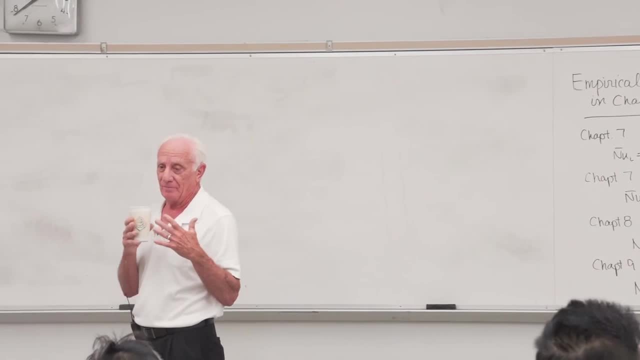 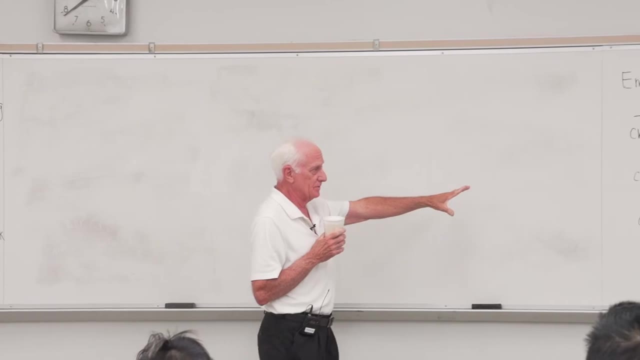 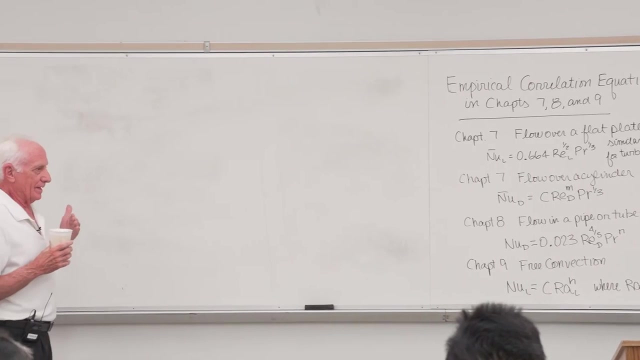 They cover more property variation and they cover more accurate data taking methods and things like that. But we in our class, we're focusing on these equations. They're the simplest ones and it's nice to start there, Okay, so now we transist to chapter nine, example nine three. 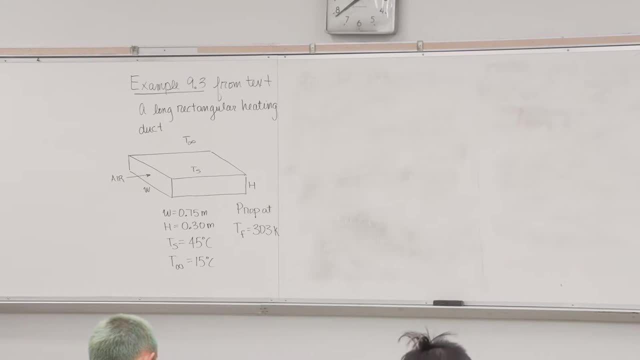 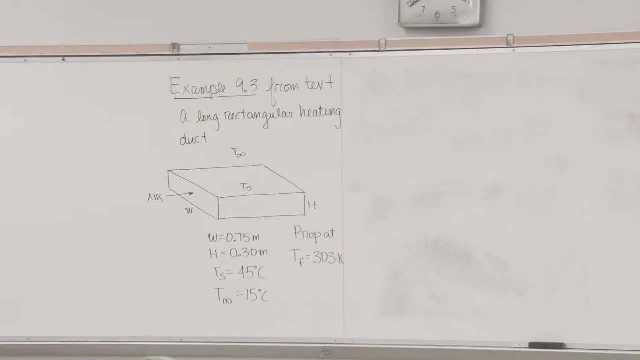 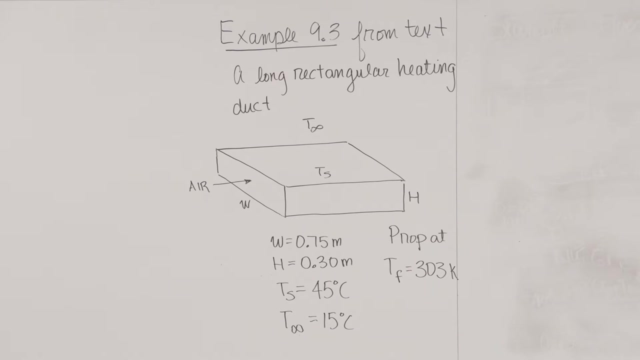 Okay, let me read it to you. The picture's on the board, but I'll read the word. I'm gonna read the words he gives you. Air flows through a long rectangular heating duct. A long rectangular heating duct. here it is. 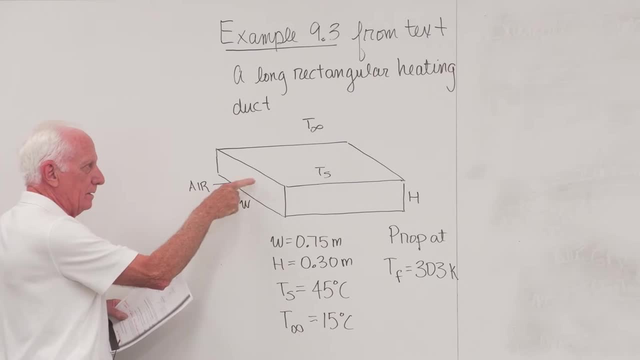 Air comes in here, left-hand side, It goes along this duct. The word is long, big giveaway: 0.75 meters wide, 0.3 meters high. The outer duct surface is at 45 degrees, So the duct surface TS 45 degrees. Keep reading. The duct is uninsulated and exposed to air at a temperature of 15, 15.. It's located in the crawl space. Now, of course, most of our homes here in Southern California that stuff's in an attic. but there are still older homes where all the duct work is in the crawl space under the floor of the home. So that's it doesn't matter. That's what he says. The temperature down there is 15 degrees, Okay. what is the heat loss from the duct? 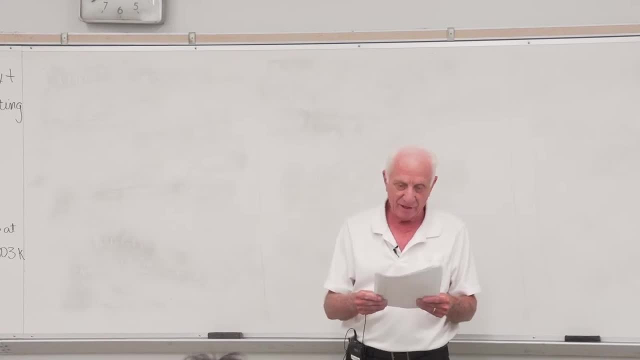 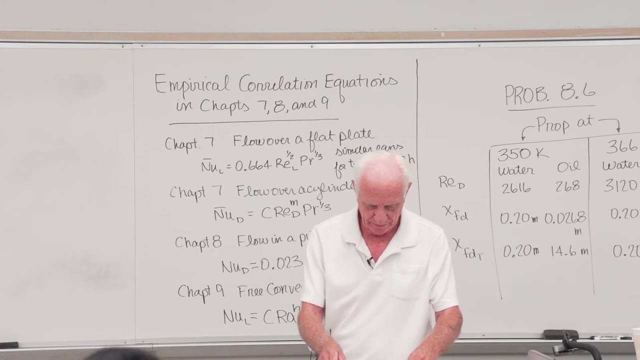 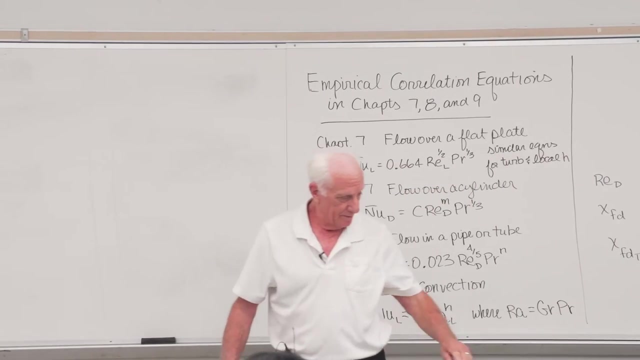 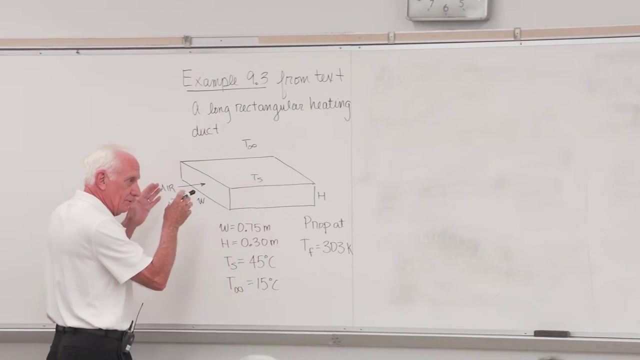 per meter of length- Okay, big hint. per meter of length, Q prime. he wants Q prime to be 15 degrees. Okay, He wants Q prime. Okay, Now I'm gonna, I'm gonna show you a picture of the duct. 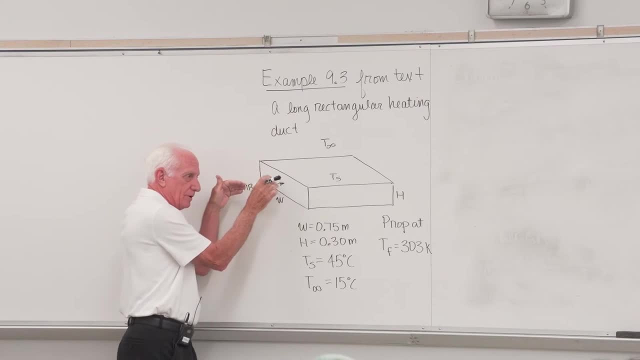 looking straight on where the air comes in, This view here on the left-hand side. Okay, the air's coming in this way from the here, Okay, so what do I see? I see a bottom surface, a top surface and two sides. 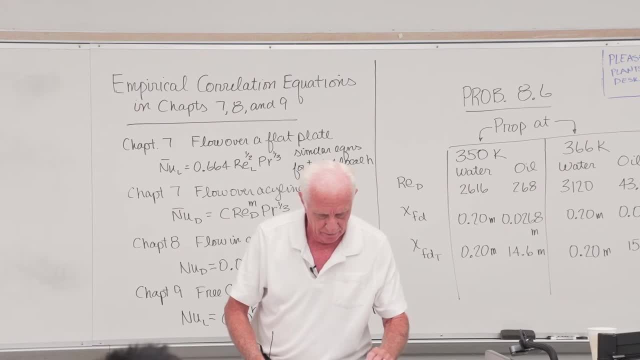 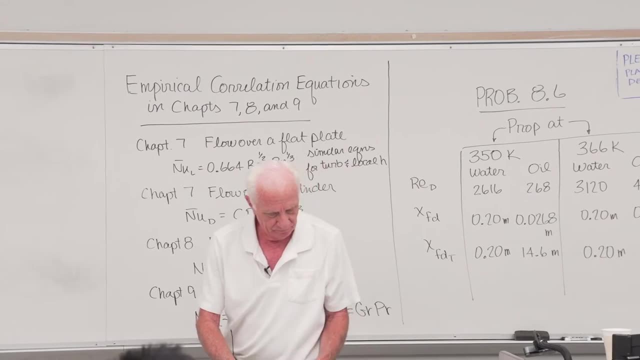 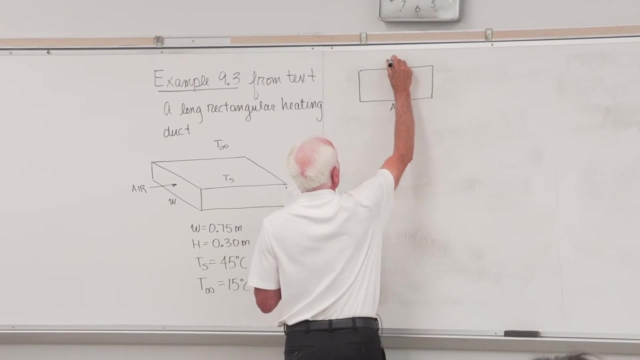 So I'm going to call those guys- I think I call that A1,, A2, and A3, and A4.. Yeah, okay, So I'm gonna call this one A1.. This is A1,, this is A2, this is A3,, this is A4. 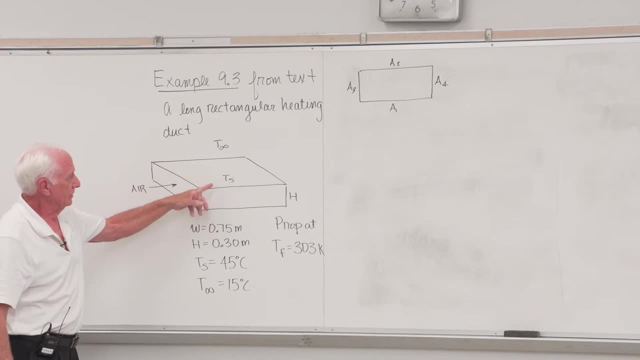 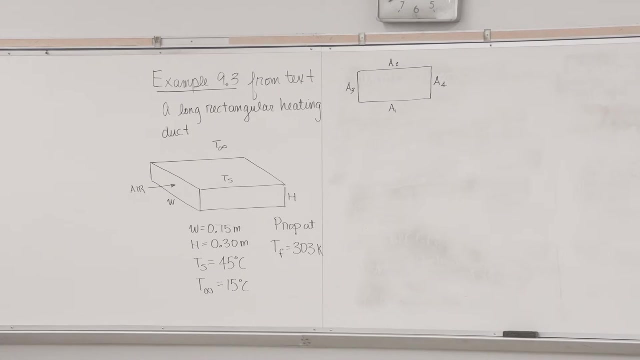 This picture here. the top surface is A2.. The bottom surface here is A1.. The left-hand side is A3.. The right-hand side is A4.. Okay, four surfaces. You can see what we've got. We've got two A1s. 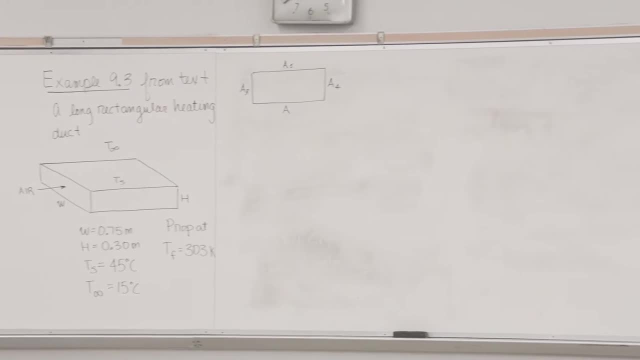 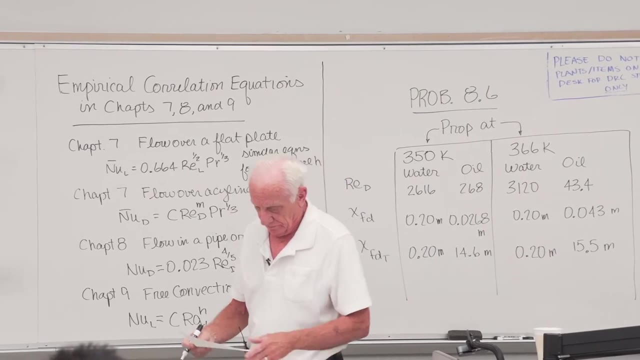 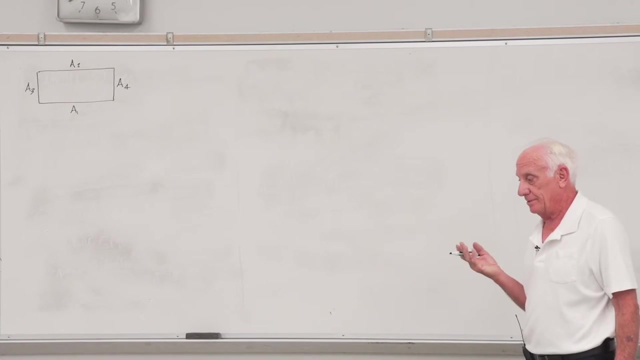 Two side surfaces, and what are they? Vertical surfaces And two horizontal surfaces, top and bottom. So now let's look at and define Q prime. We need H- okay, Define H. we need Rayleigh- Okay, we'll do that. 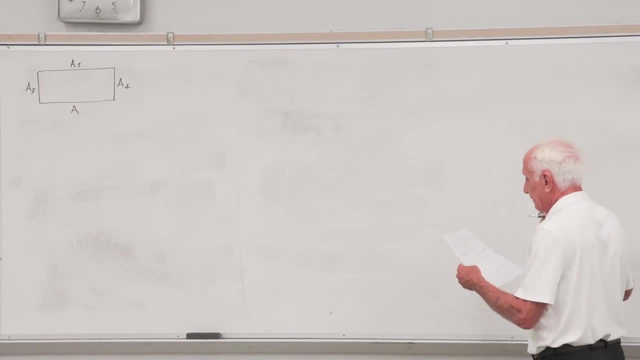 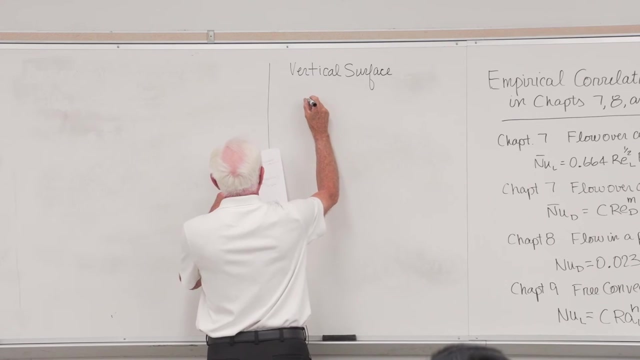 But let's start out and summarize again what we did last time for a vertical surface: Okay, vertical surface, Equation 924.. Laminar R: turbulent Magic number Rayleigh one times 10 to the ninth Horizontal plate: Okay, two possibilities. 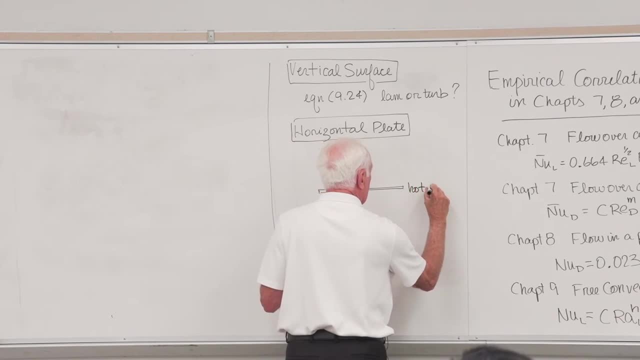 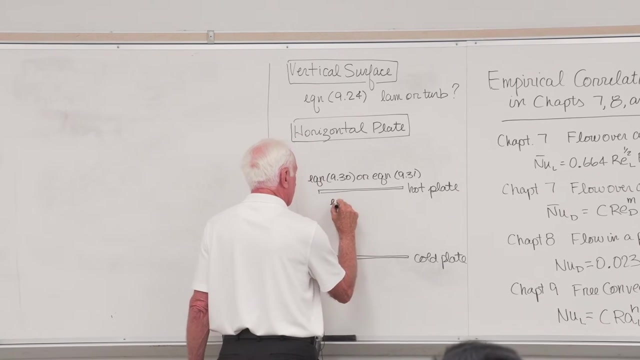 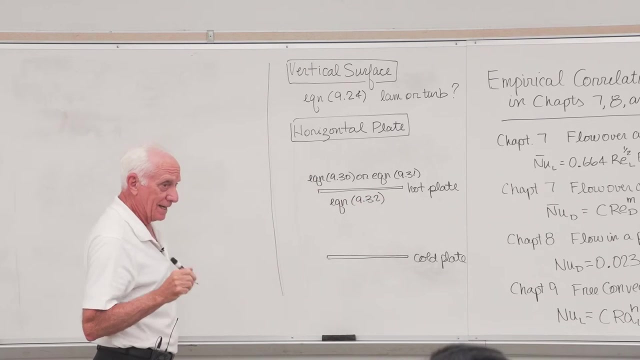 A hot plate And a cold plate. If it's a hot plate and you look at the top surface, use either equation 930 or equation 931.. The bottom surface of a hot plate: use equation 932.. If it's a cold plate and it's the top surface, use equation 932.. 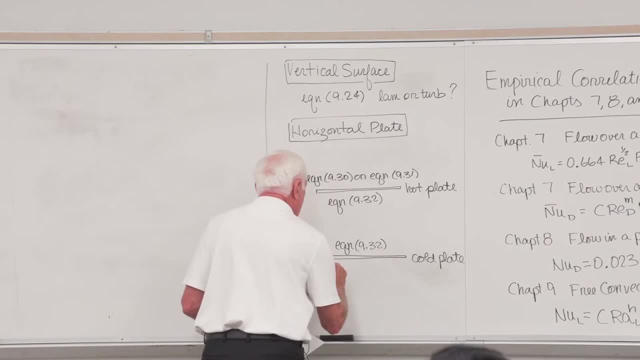 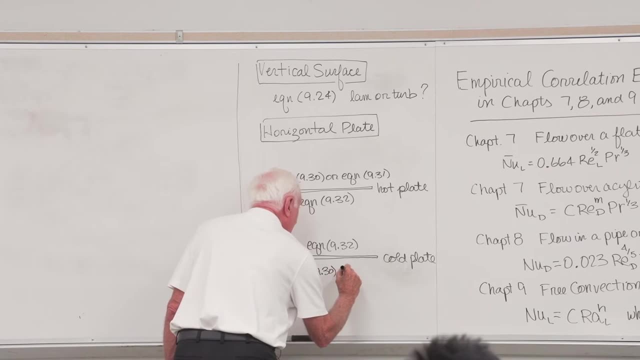 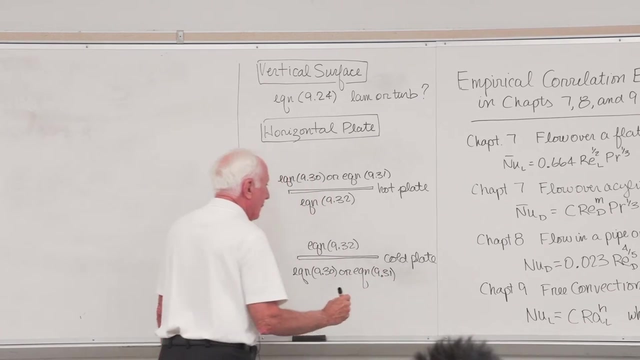 If it's a cold plate and it's the bottom surface, use equation 930 or 931.. If it's a cold plate and it's the bottom surface, use equation 932.. If it's a cold plate and it's the bottom surface, use equation 932.. 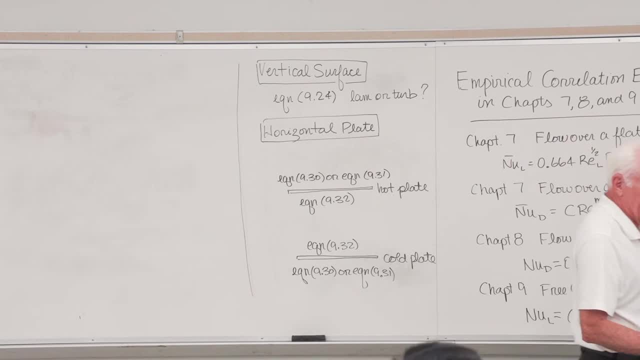 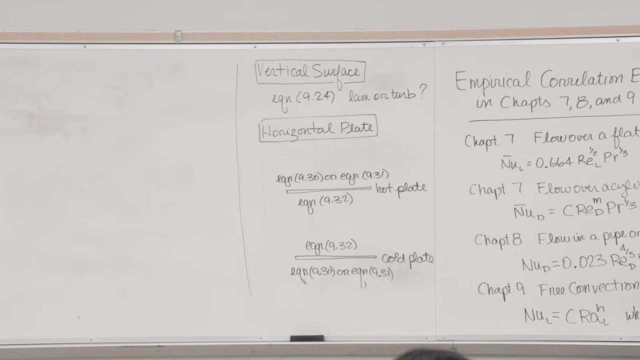 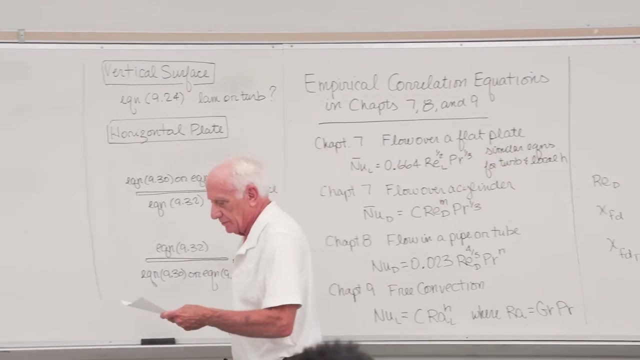 Okay, so there's our choices. So now we look at what we've got over there on our uninsulated duct. All right, let's do the vertical surfaces first. So these are the two side walls which should be for A3 and A4 vertical surfaces. 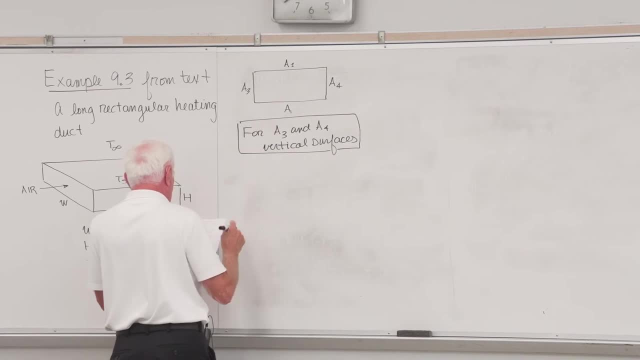 Okay, we'll start out. TF, the film. TF, that's the film terrestrial ferrule. Okay, temperature 303 K, that's T surface plus T infinity divided by 2. get your properties at that temperature. chapter 6, 7: first step: calculate Reynolds number. 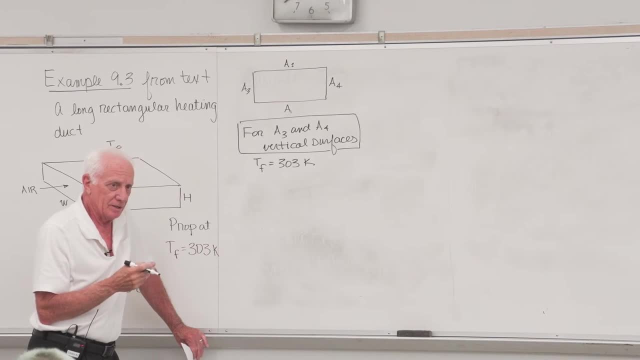 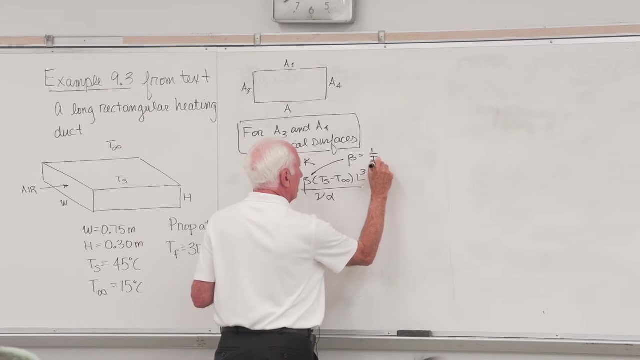 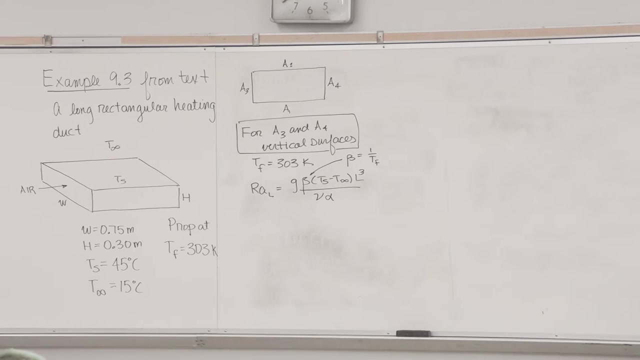 if you can, chapter 9, first step: calculate the Rayleigh number. if you can, okay, the Rayleigh number L G beta L cubed divided by nu alpha G: 9.81 beta. beta 1 over T, film 1 over 303, you got a shift gears. if you're in chapter 7, L means the 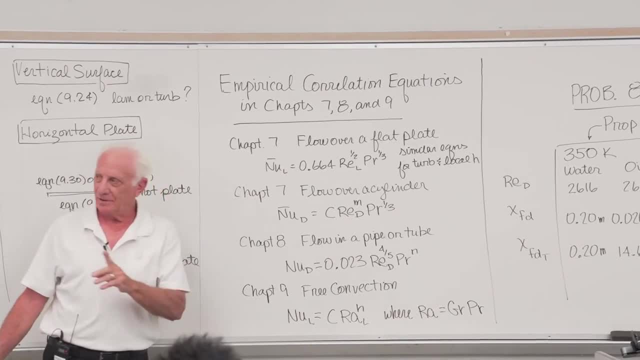 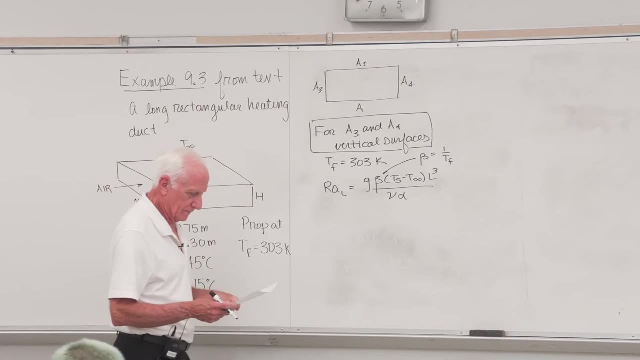 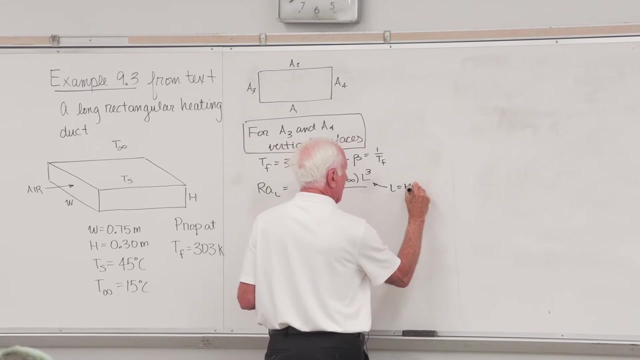 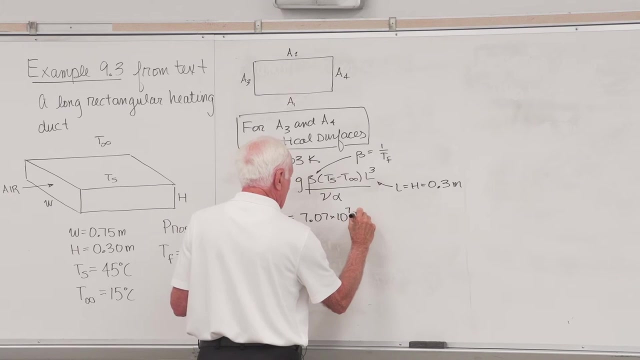 horizontal length of the plate X equal L, if you're in this chapter, of course. L means what it's: the vertical surface. so L is the height H, so L is 0.3. put all those guys in there. get really 7.07 times 10 to the seventh, less than the. 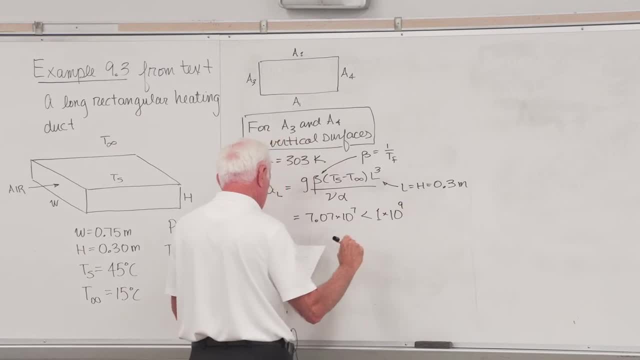 magic number: one times two, 10 to the ninth, so it's laminar. okay, so now we know when I go to that equation for vertical surfaces it's going to be laminar flow equation. equation 924- all right. equation 924, Nusselt, based on the length, L, C, Rayleigh L to the end, C. 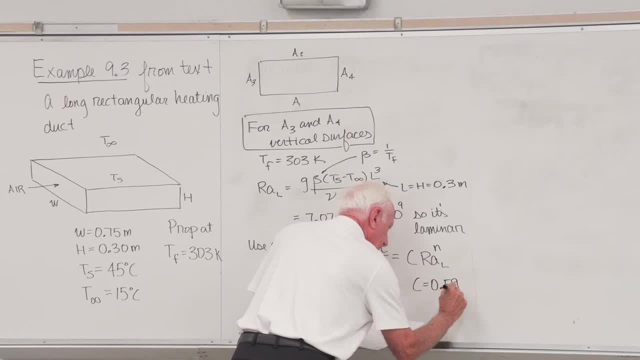 0.59 for laminar flow and 1: 4th for laminar flow solved to get H 4.77. okay, so that gives us now a start. we've got area a three and a a four, and So now we're going to do area a1, area a1. 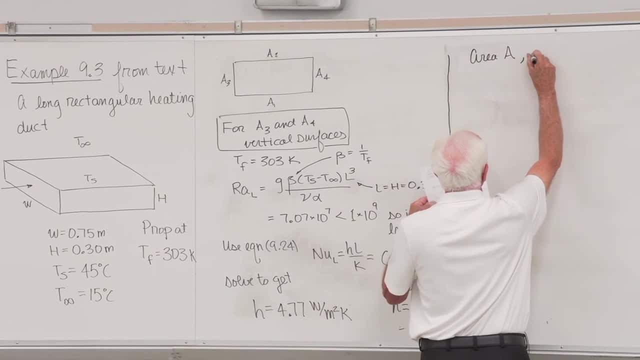 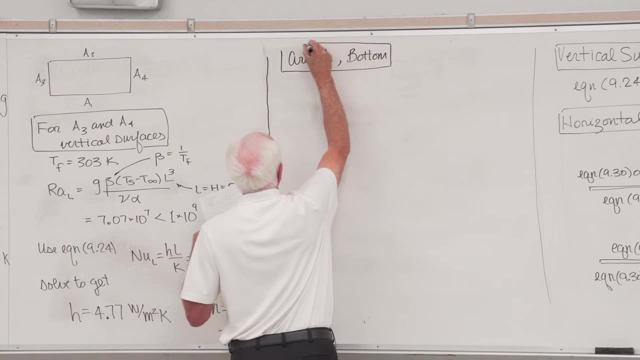 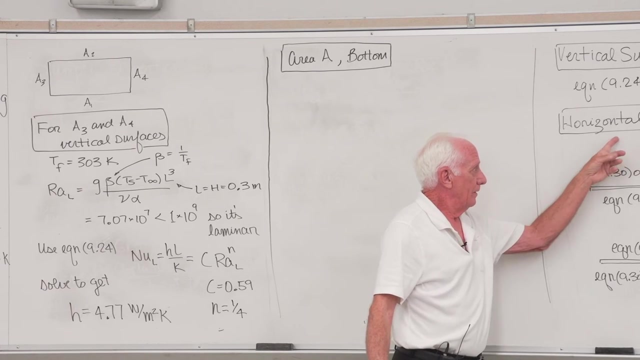 So area a1 is the bottom Horizontal plate. There's a plate hot or is it cold? Oh, you can see TS is 45. It's hot hot plate Is at the top or the bottom of the heated hot plate? the top. Okay, Got it. 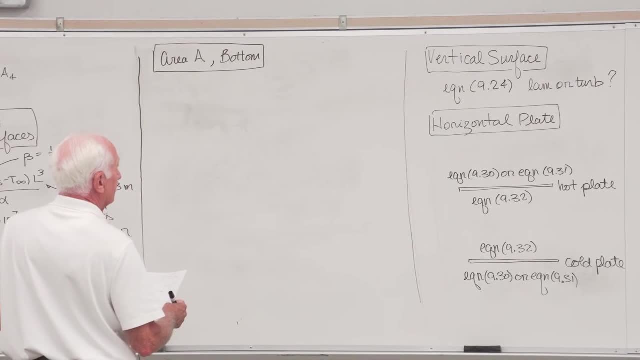 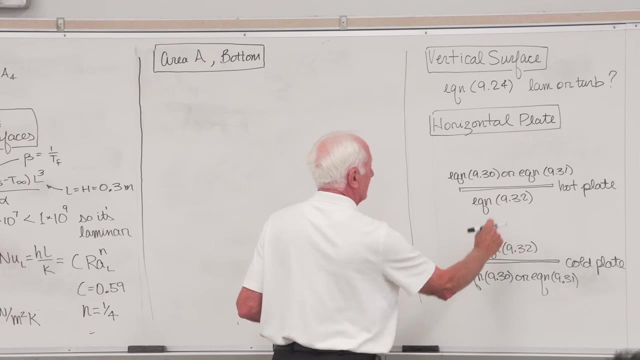 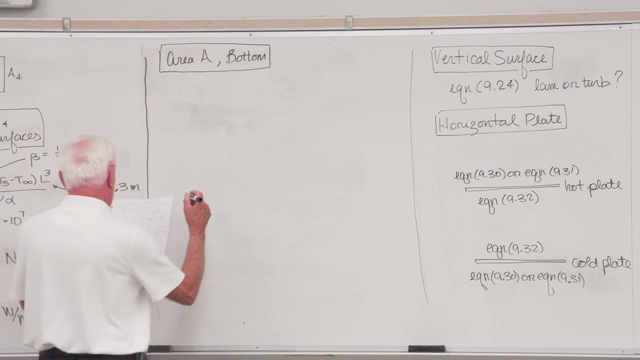 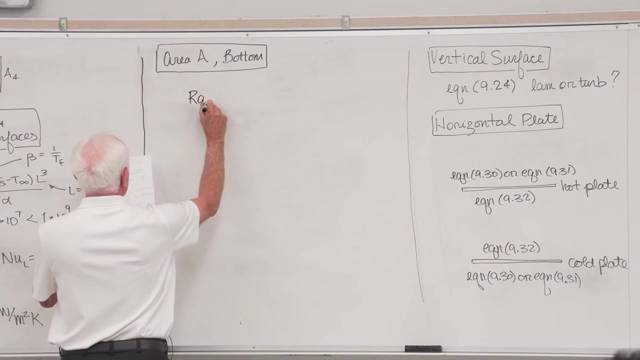 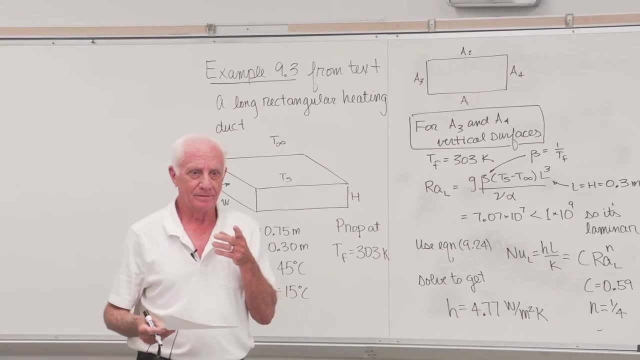 Well, this I'm doing it, I'm doing the um. Okay, let's see the bottom plate. so we're doing the bottom plate. There's that guy there, heated plate, bottom 932. First step: find a really number buds. Of course. my problem now is: what's el? 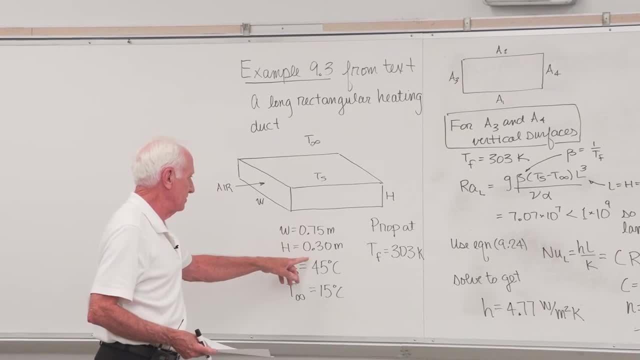 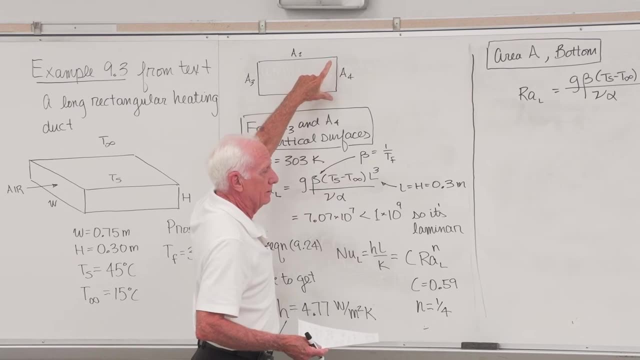 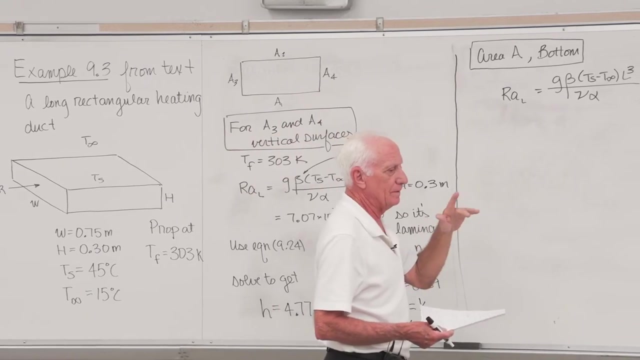 Is it length of something I don't know? is it point seven, five meters? is it point three meters? What's el Vertical service? I knew L, That's L, right there Is the horizontal surface, this guy right here? No, It's not that guy, It's in your notes from last week's lecture. 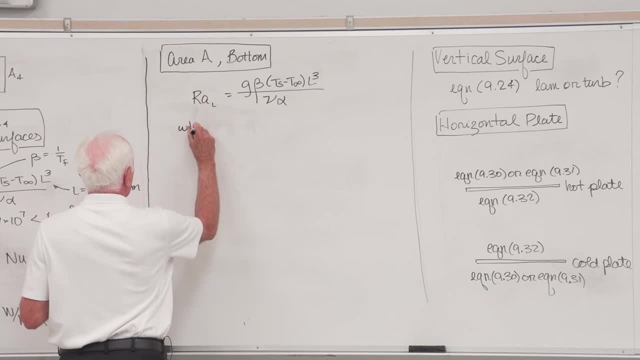 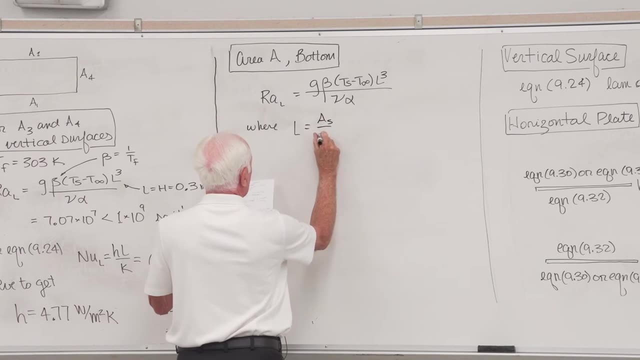 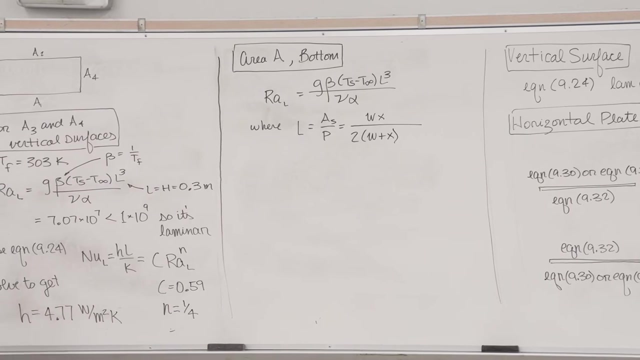 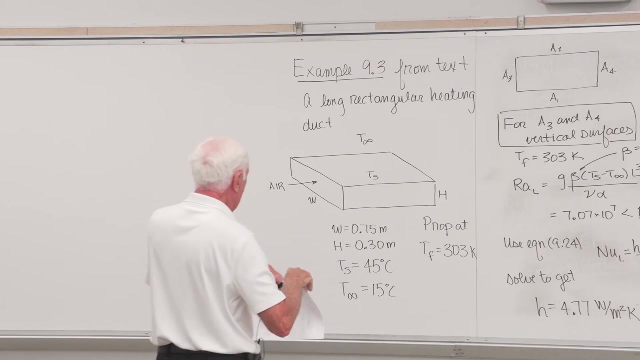 from last time. it says: where L is equal to the surface area divided by the perimeter. surface area, W times X, perimeter 2 times W plus X. and my problem is, of course, I don't know what X is. I did what is X? X is the distance. 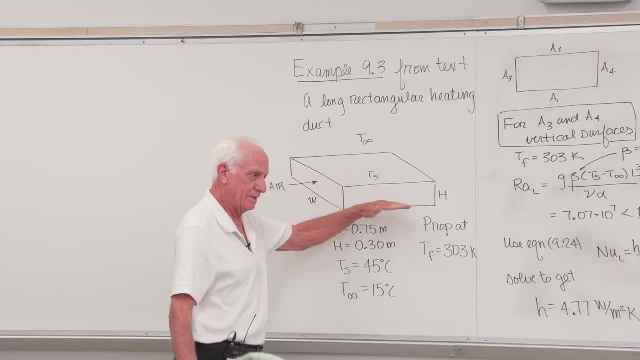 measured along word. this is that the air is flowing, the heated air flowing. this is X. I don't know X, but he was kind. he said: oh, by the way, it's long, oh, thank you. so I'm just gonna put X in the equation. I mean, I don't know what it's. 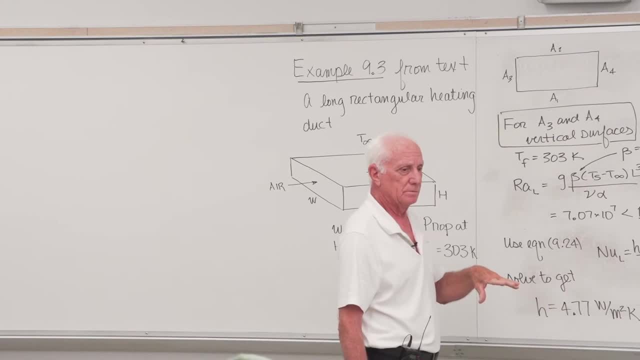 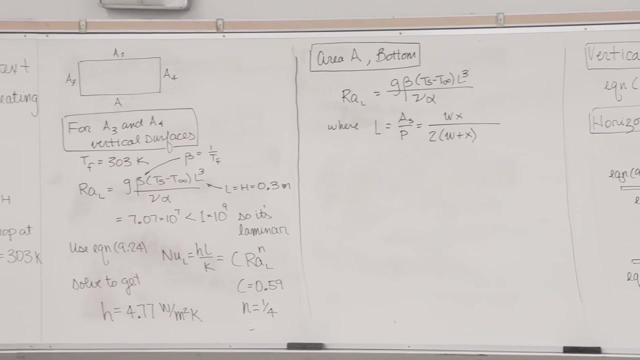 gonna be a big number. I know X is gonna be a big number, you, okay. so now I say to myself: you know what this parentheses? W plus X. X is a real big number. W is probably a real small number. watch W- 3 tenths meters, how. 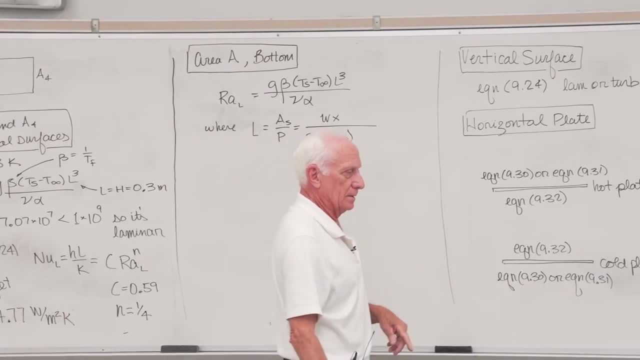 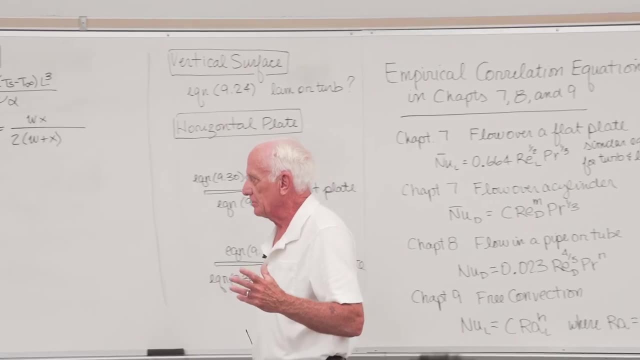 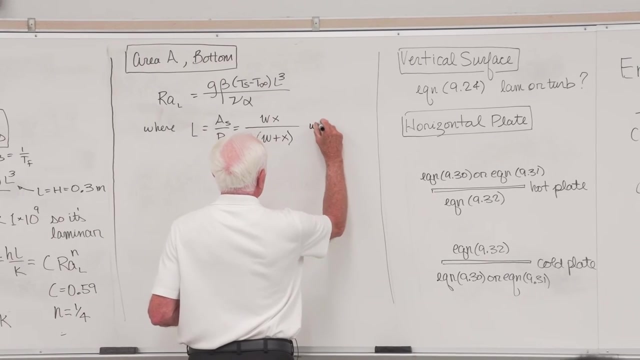 long is this duct in your attic or in your crawlspace? what's 50, 50 feet, 20, 30 meters. 20, 30 meters, meters, 30 meters. anyway, you're making this because you're not going to make more squared months. can't always know. before did I say thisboard, this deflation? 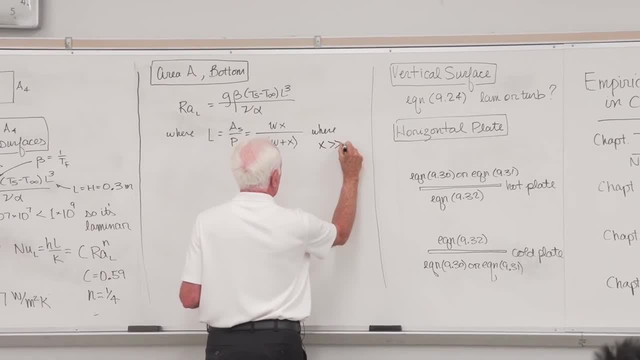 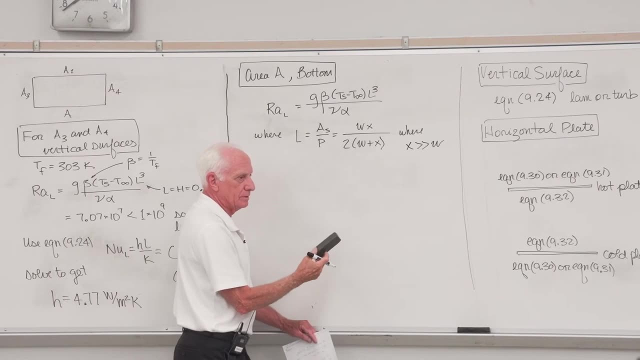 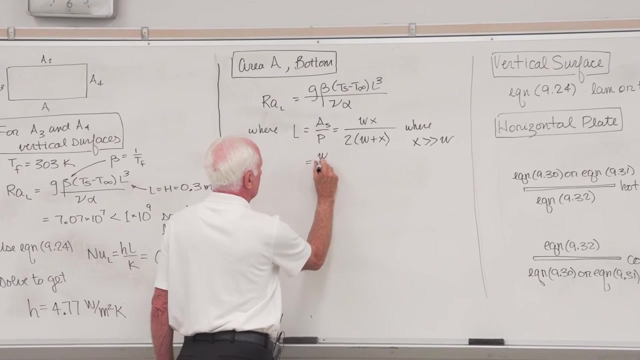 why in the world did you say this? please remember what it's about. уждate, good reference century. in a little more here the form, just for you to be able to concentrate on this: how toama noted how to Sydney, Sir. 2019. Wx over 2x. okay, L is W over 2.. 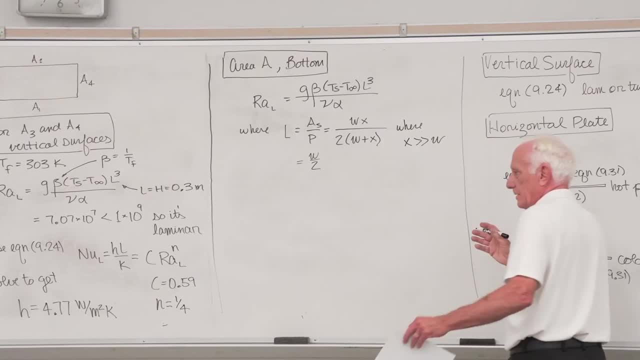 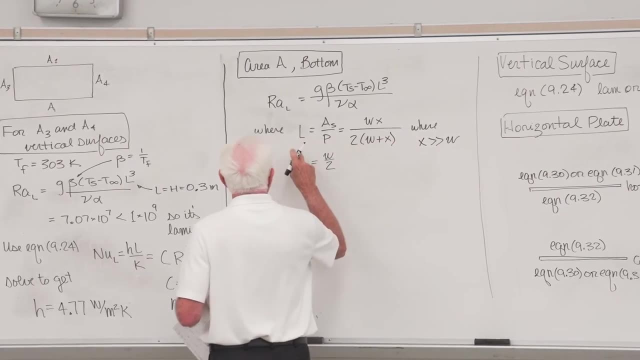 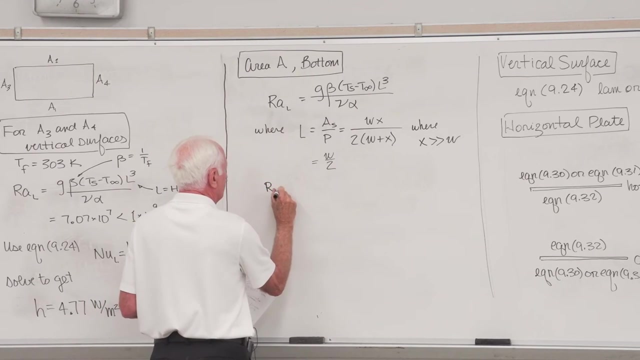 An approximation. the bigger the length of the duct is compared to W, the better the approximation. but that's what you do. So now you can get the Rayleigh number, because you know L is W over 2.. Okay, so Rayleigh number then, based on L, comes out to be 1.3810 to the 8th. 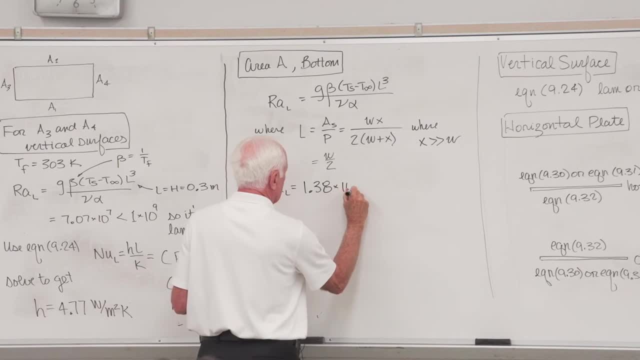 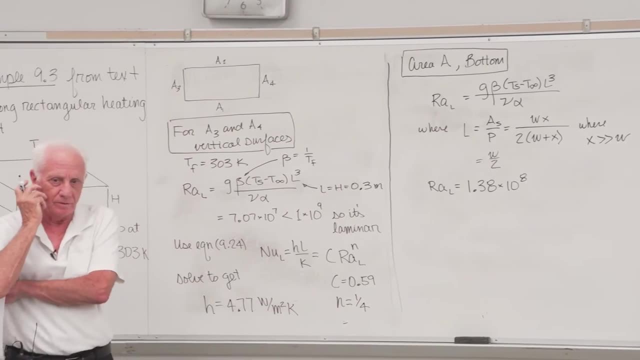 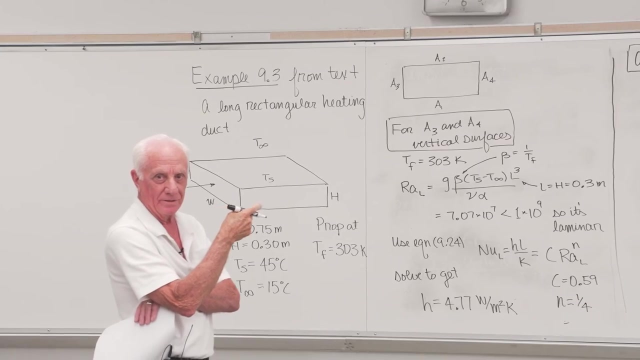 1.38 times 10 to the 8th. Does that mean it's laminar flow? No. Turbulent flow- No. What does it mean? I don't know and I don't care. That's the number it is. That's what it is. 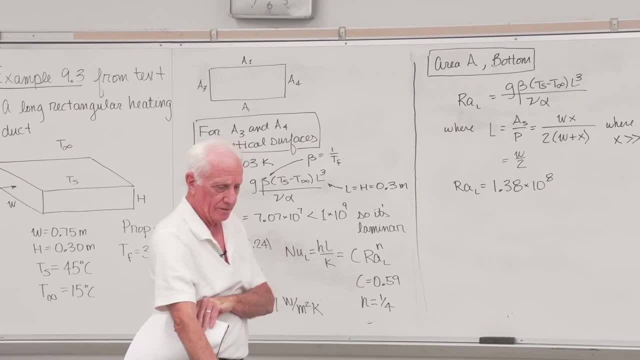 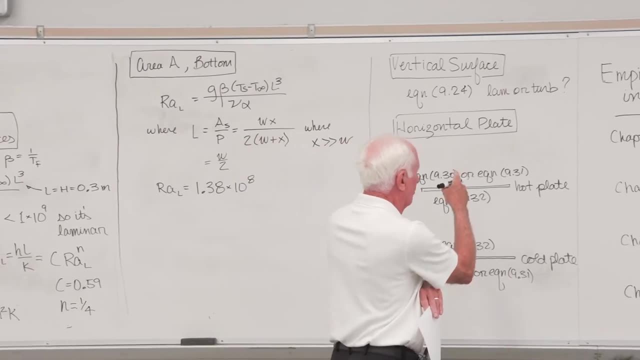 When air rises off of the floor, for instance, is that laminar flow of air off the floor turbulent flow? No, it's not a boundary layer. on a vertical plate It's not a boundary layer. So you don't ask questions like that. 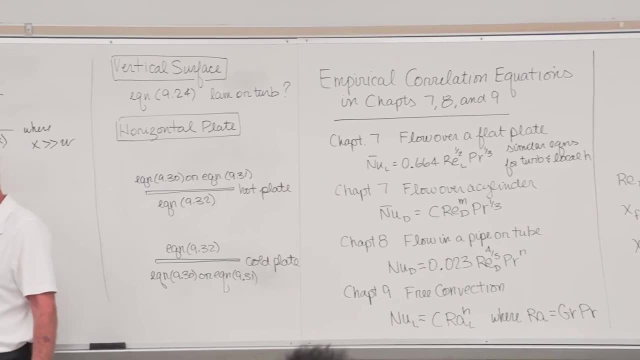 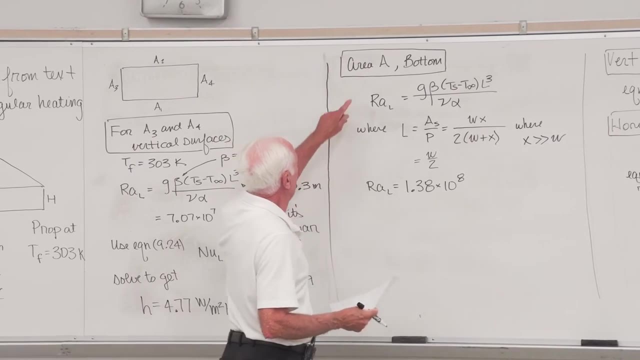 You ask questions over here like that: Is it laminar or turbulent? Here you don't ask questions like that. You use it in what? The equation: Which one? Bottom, heated plate, hot plate, bottom 932.. 932.. 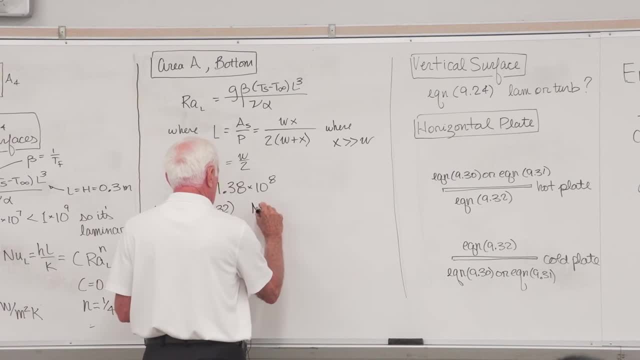 Okay so 932.. 932.. 932. 932. 932,. we have Nusselt L HL over K 0.52 Rayleigh number raised to the one-fifth power. This gives H equal 1.56.. 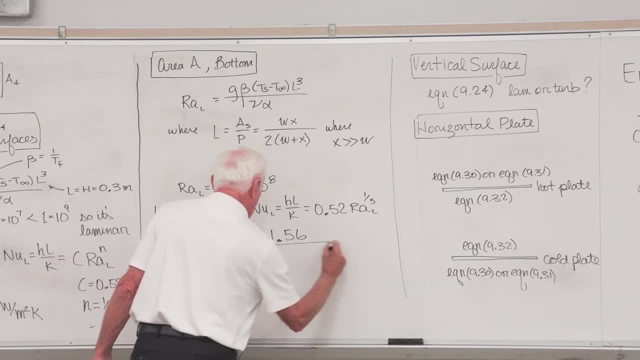 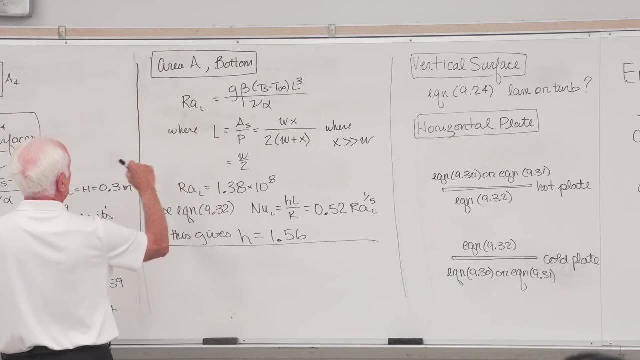 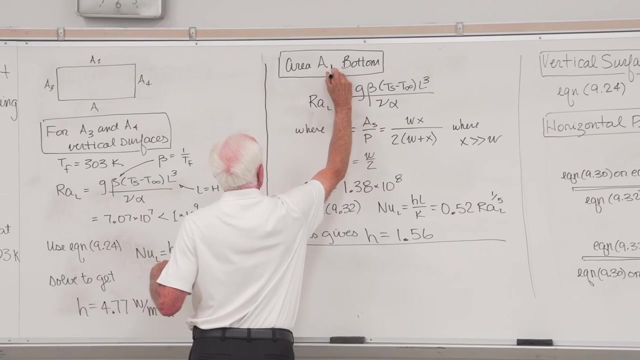 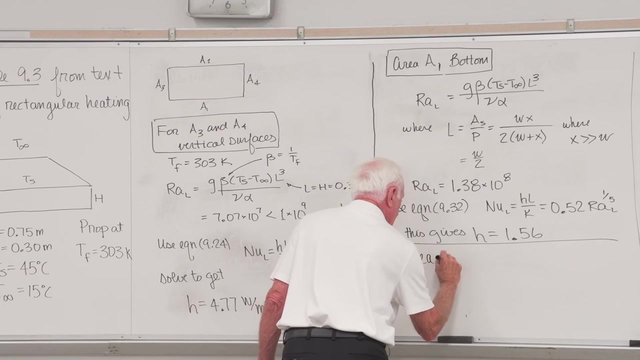 Okay, one more to go Area. oh, that should be. yeah, this is the bottom, so area A1.. Now we'll do area A to the top. Okay, did L change? No, it's the same rectangular area. 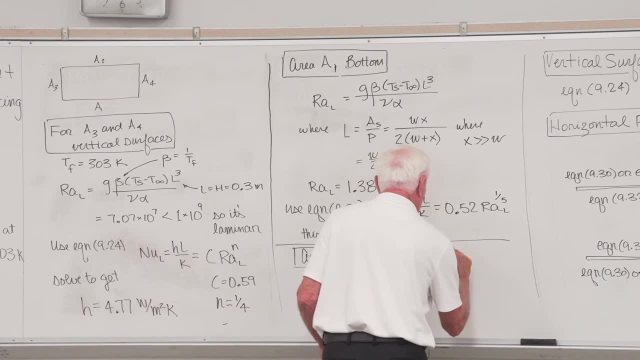 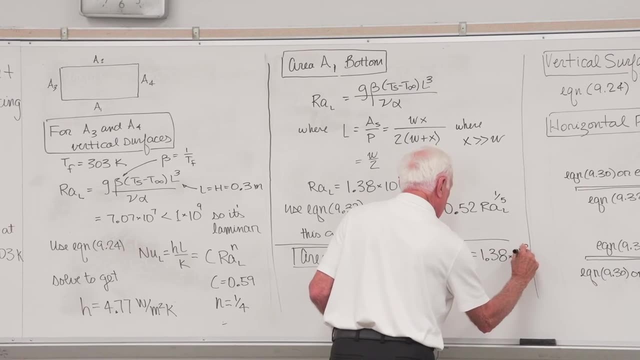 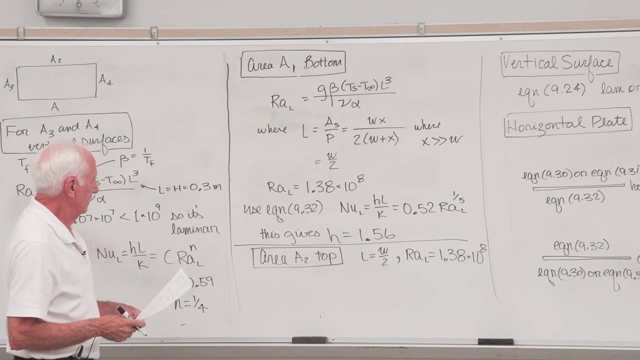 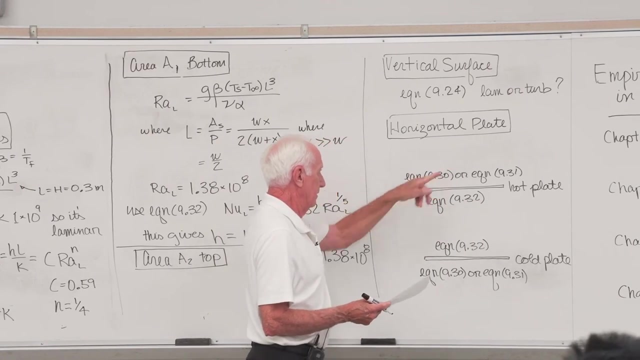 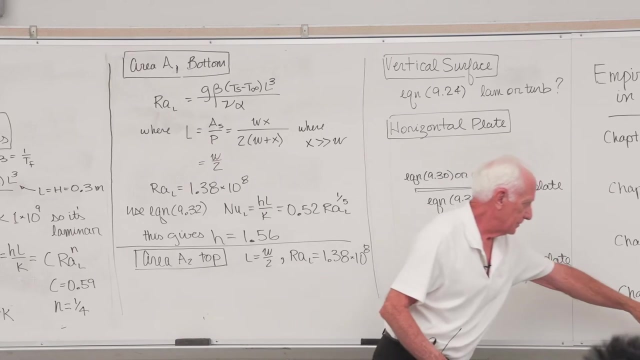 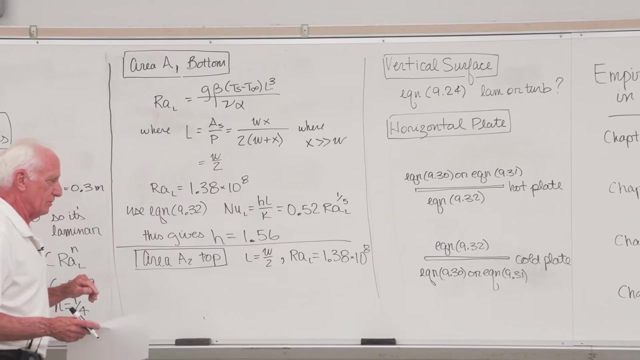 Did the Rayleigh number change? No, it's the same. Did the equation change? Of course it did. Okay, heated plate. Heated plate here, Top surface, top surface. here There's a table. There's a table that gives you C and N depending on where you are on the Rayleigh number. 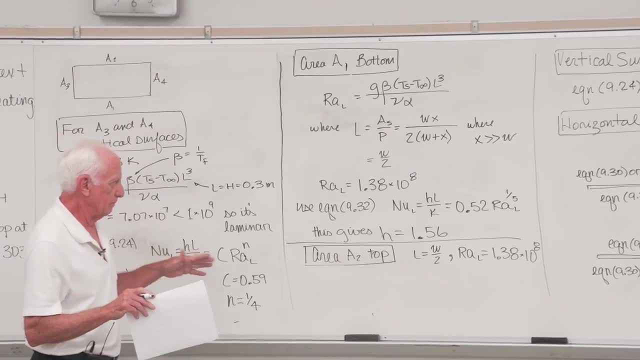 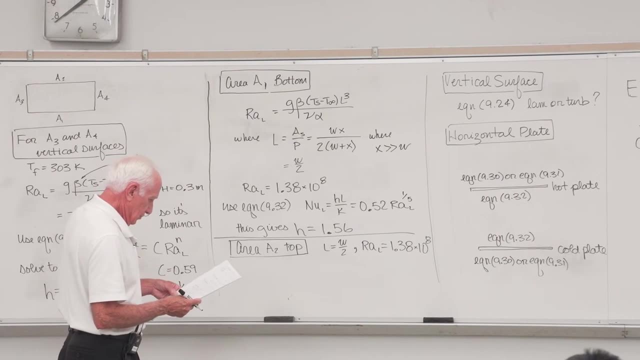 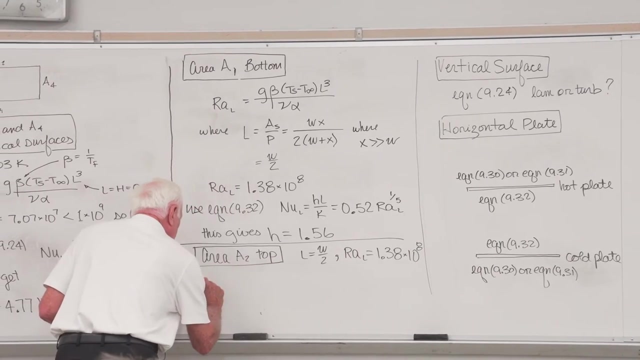 Two ranges. There's two values of C and N, depending on where the Reynolds Rayleigh number falls in the range of values given in it. So I'll put them down here. This is equation 931.. Yeah, top equation 931.. 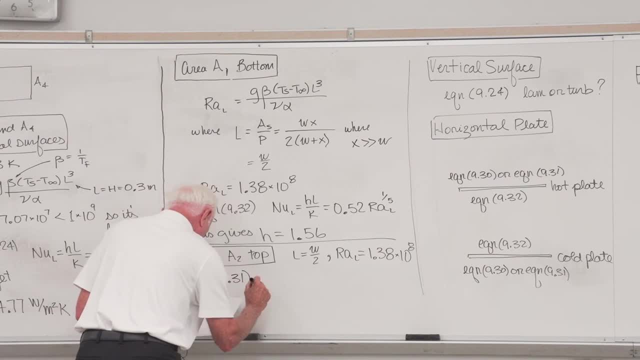 No salt. No salt: L 0.15 Rayleigh L raised to the power one-third. This gives L 0.15 Rayleigh L raised to the power one-third. This gives 0.15 Rayleigh L raised to the power one-third. 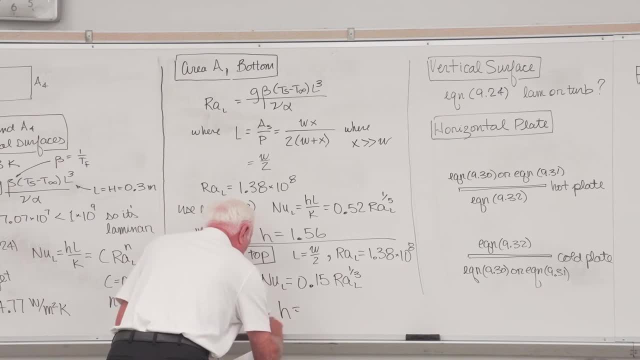 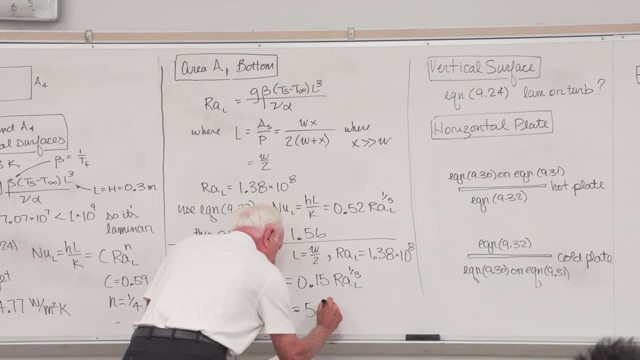 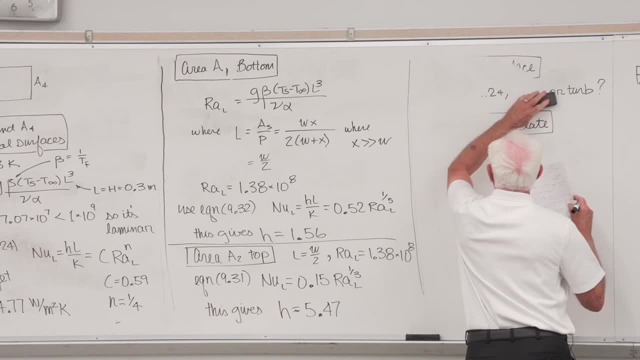 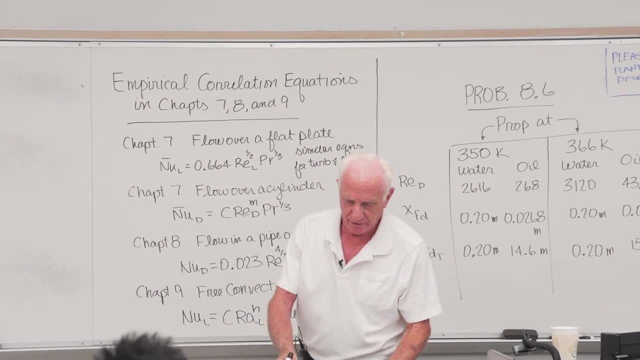 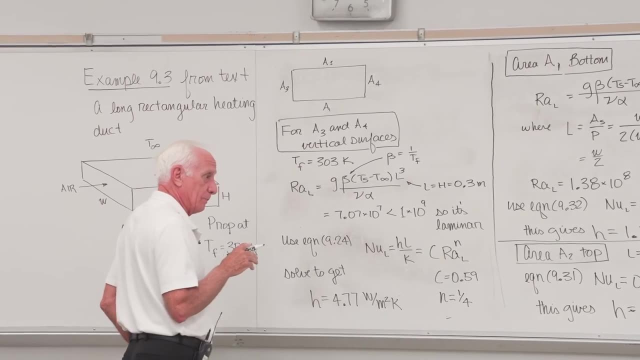 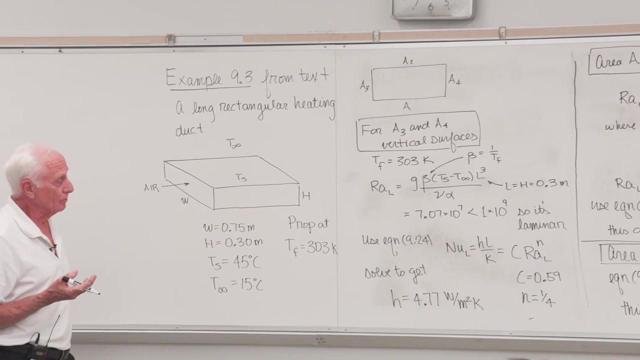 This gives. We have H for each of the surfaces: A1, A2,, A3, A4.. Would you expect the best heat transfer? You don't want the heat transfer. You want to keep the air in the duct warm, But where does most of the heat transfer take place? 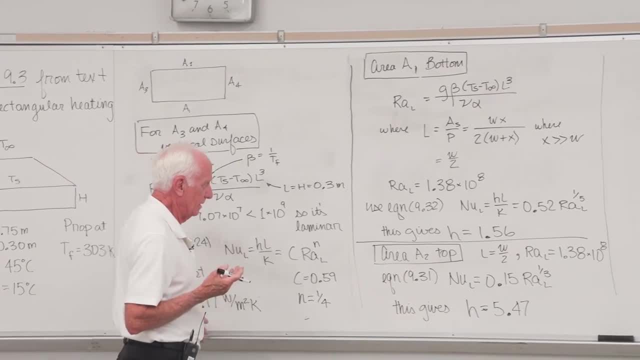 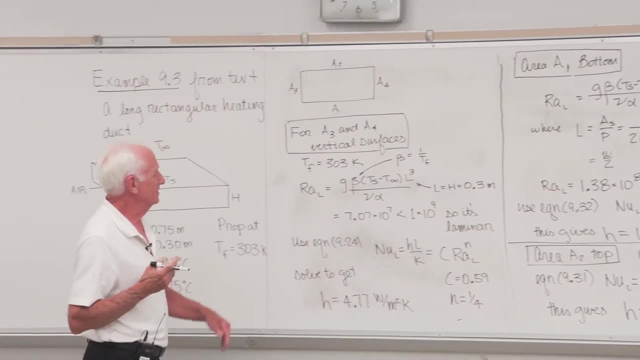 Oh, look at the H's 477,, 156,, 547.. There he is, the top surface. Of course it's the top surface. You've got air being heated near the top surface and it wants to go up. 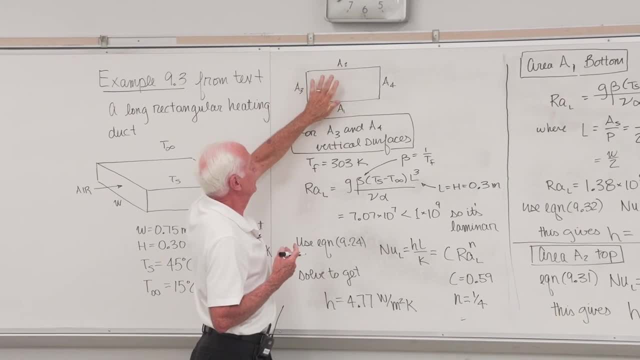 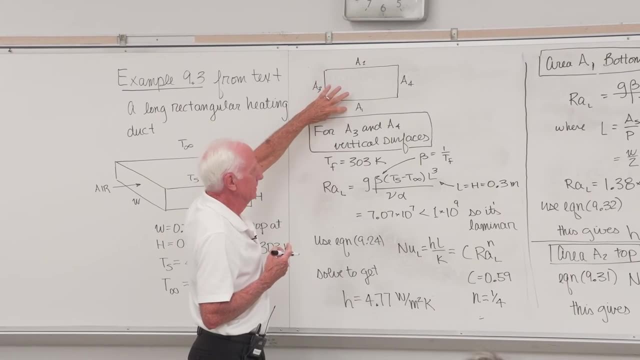 Its density goes down. the buoyant force goes up. it wants to raise up, That's fine, nothing stops it. it can go straight up. A1, the bottom surface. The colder air touches the surface, it gets heated buoyancy. it wants to go up. 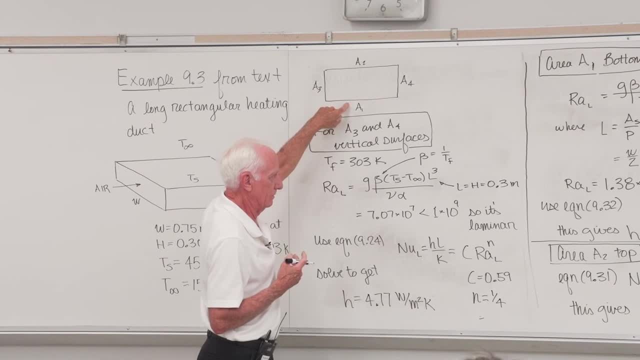 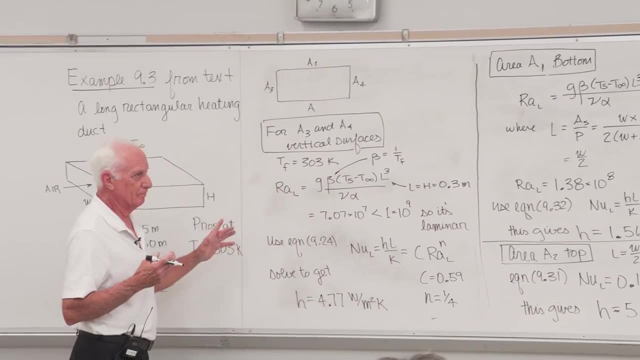 It can't. there's a wall. Bad heat transfer. oh yeah, real bad heat transfer. Real good heat transfer Somewhere in the middle on the sides. boundary layer, boundary layer builds up here. boundary layer builds up here. 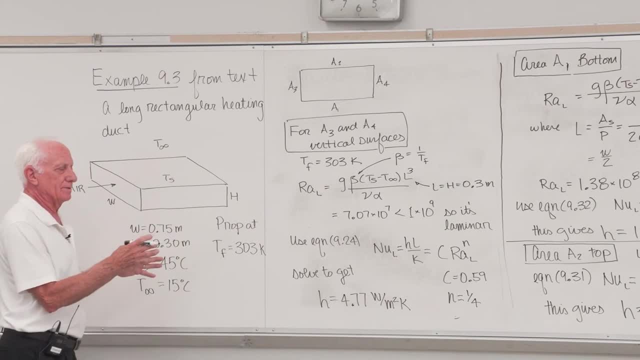 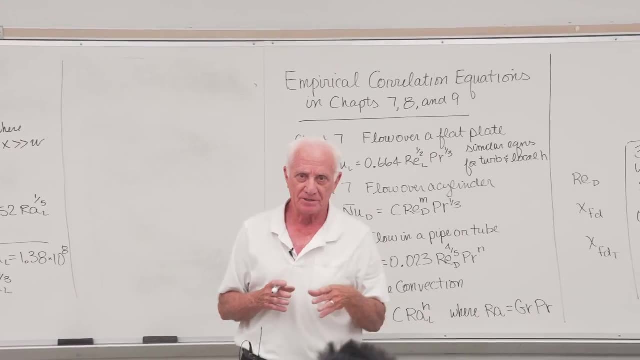 What is it? laminar boundary layer. So yeah, it makes sense. It's always good when you get answers to see if it makes some physical sense to you. If it doesn't go back and check your properties, Most errors are in those properties. 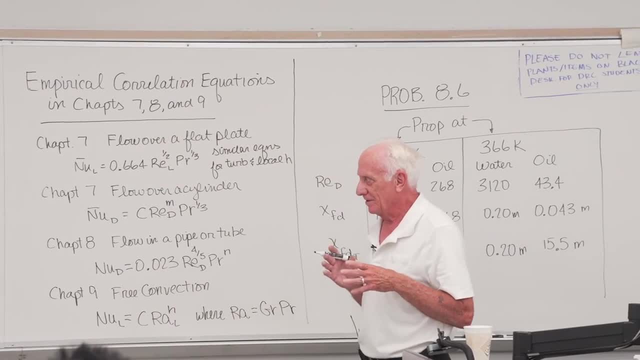 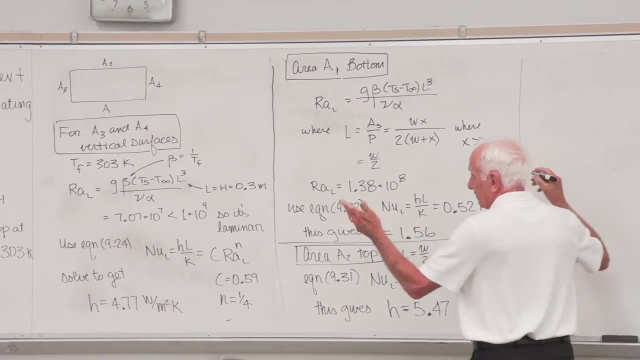 People get the powers of 10 wrong many times, But that's generally what happens. Okay, now we're not done. We've got the H's, now you've got to find the Q. Okay, that's the problem set: Find Q prime. 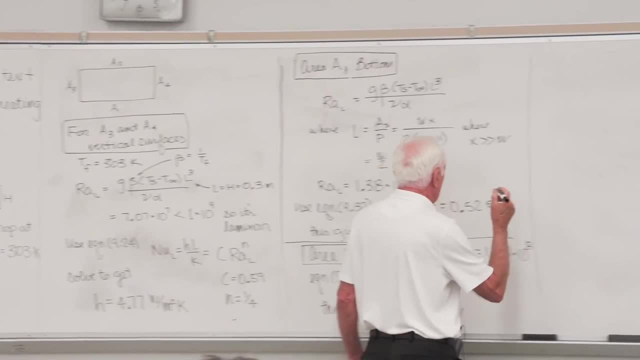 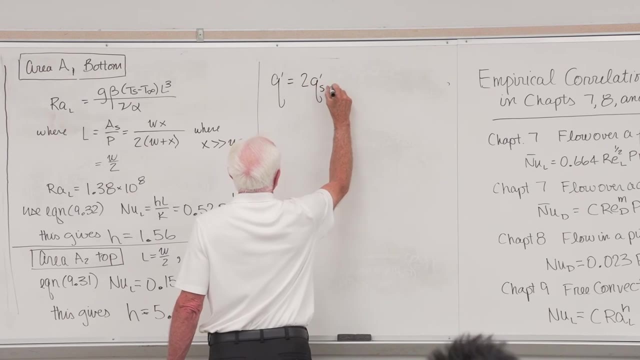 Watts per meter, because I don't know the length. Okay, so Q prime equal. there are two sides Q prime sides plus. there's a top Q top plus. there's a bottom Q bottom prime prime. Okay, let's do this guy first. 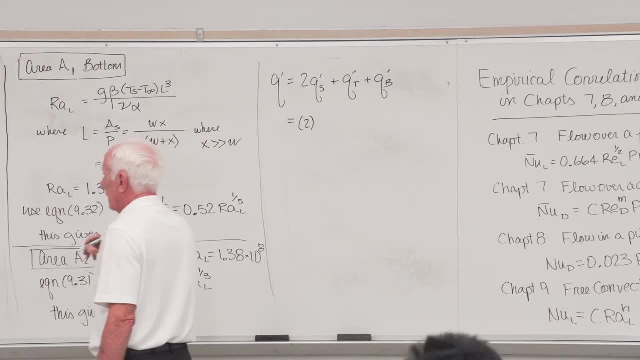 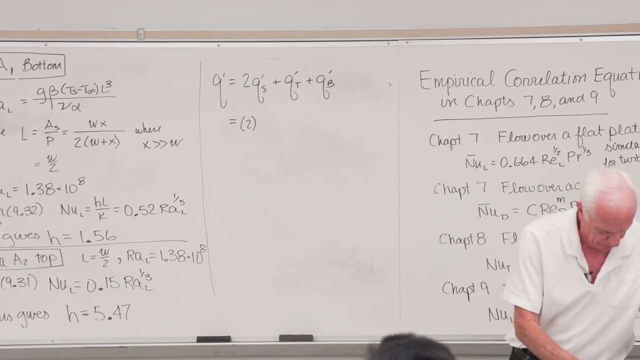 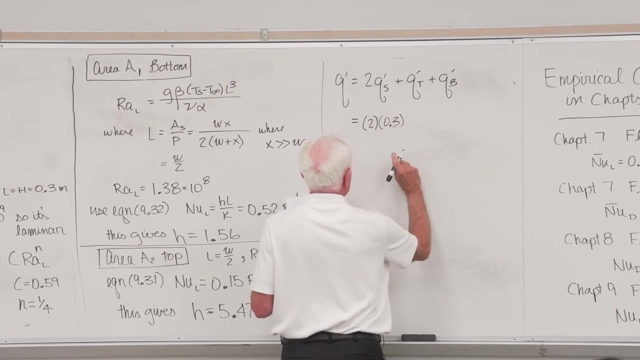 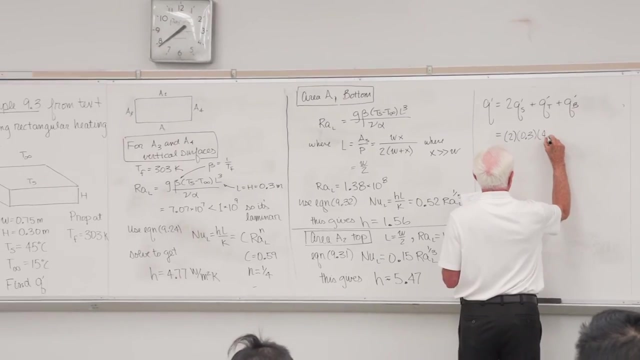 Two: The. this is for the sides. Okay, the sides have H, So the two sides 0.3.. That's the height of the side And the H is 4.77.. 4.77. Plus big brackets. 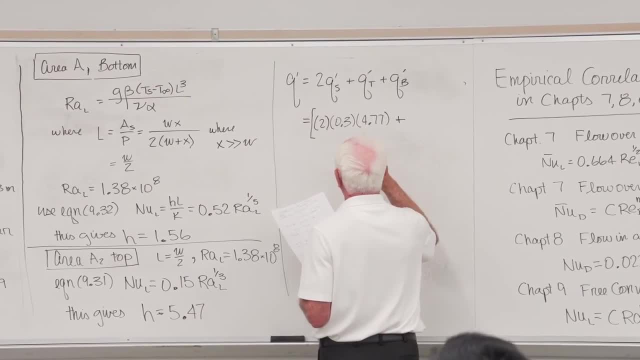 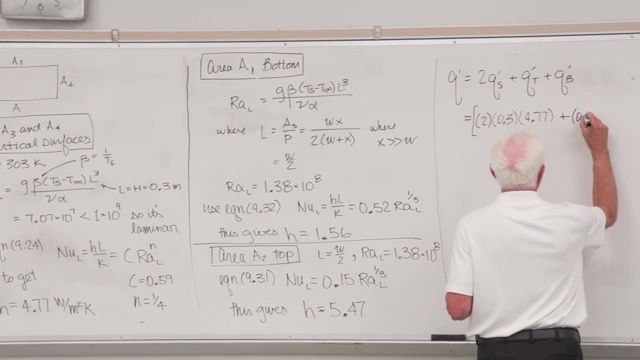 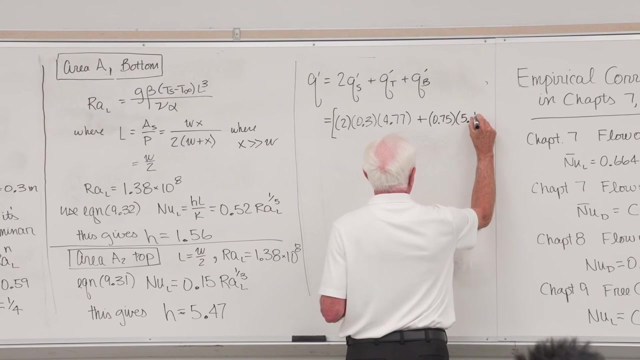 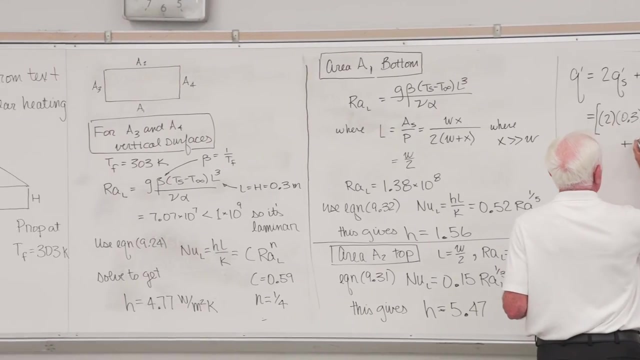 There big bracket. The top For the top W is 0.75.. H for the top 5.47.. Plus the bottom, 0.47.. That's W of 7.5, pardon me. 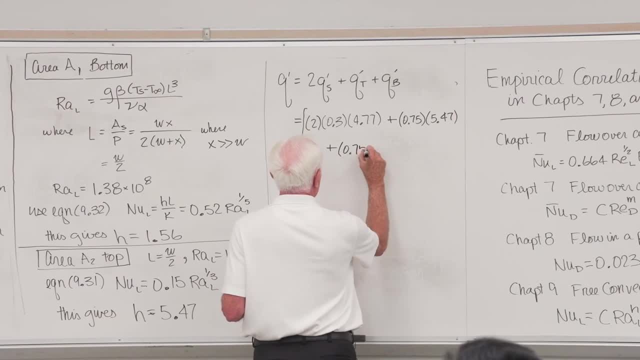 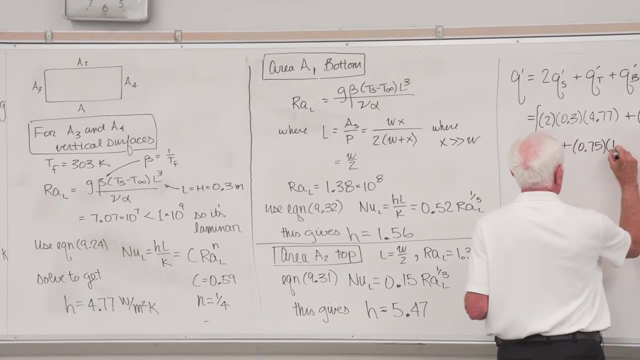 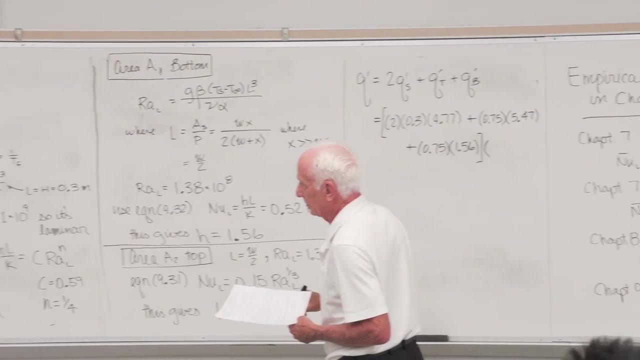 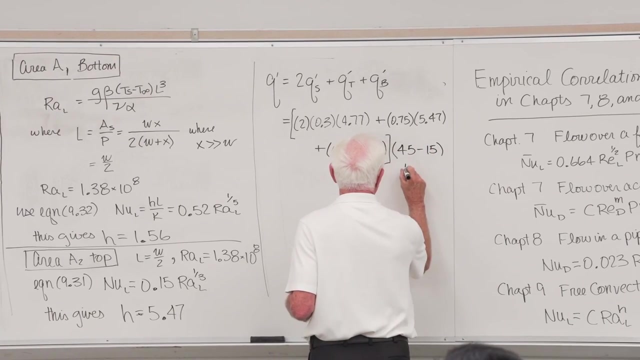 H on the bottom is low 1.56.. H A delta T: Okay. delta T: hot minus cold, 45 minus 15.. Okay, So Q prime Q. prime H on the bottom is low, 1.56.. 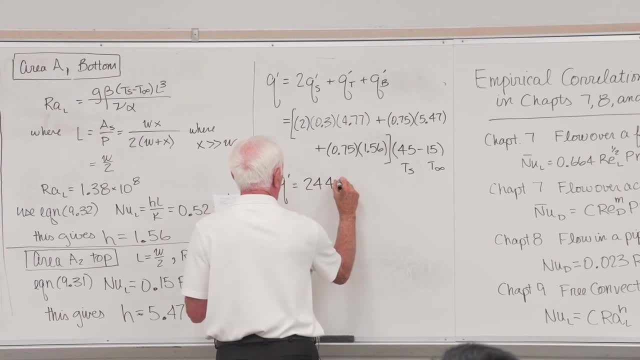 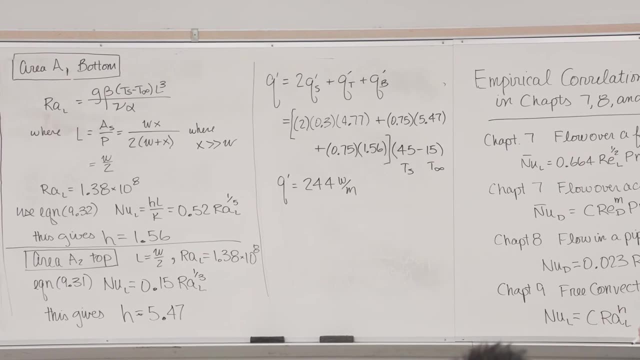 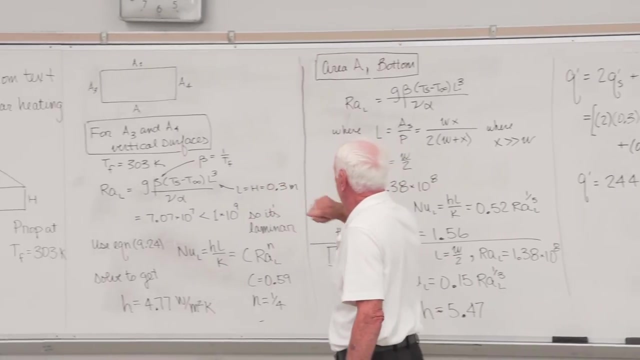 Comes out to be 244 watts per meter. Comes out to be 244 watts per meter. Okay, so that covered three equations. Okay, so that covered three equations. Vertical surfaces, Got it. Horizontal surfaces: Here's a key point. 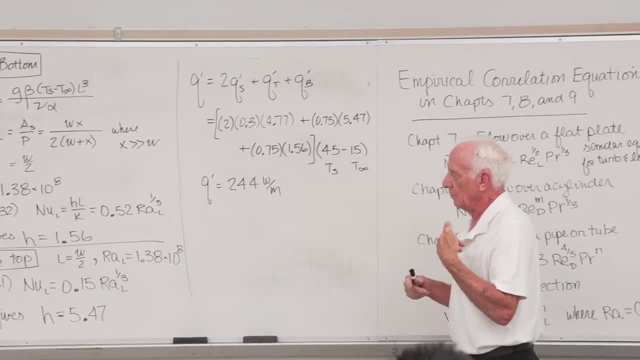 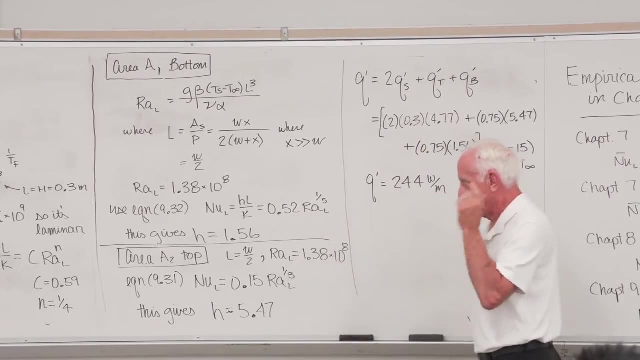 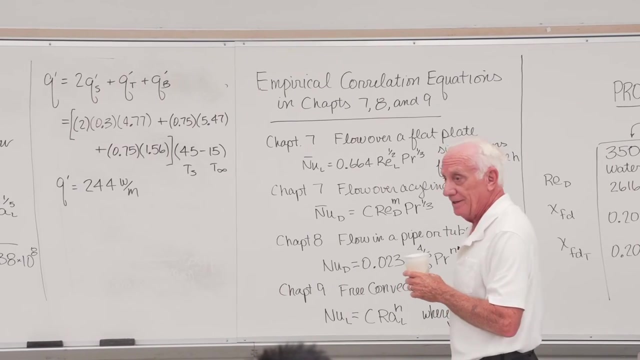 This here. Let's go lots of more. This here needed. got it. Top surface- one equation. Bottom surface- other equation. Here here. So that example problem is a good one because it covers all of those possibilities in there. 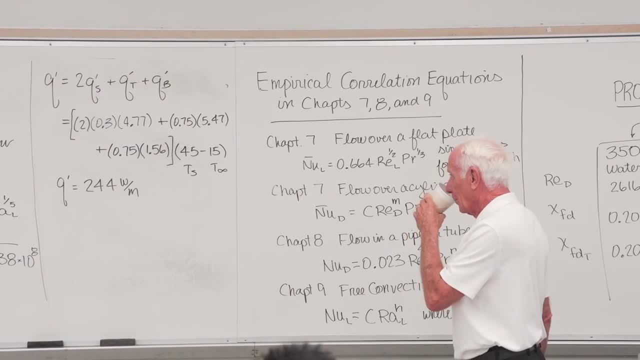 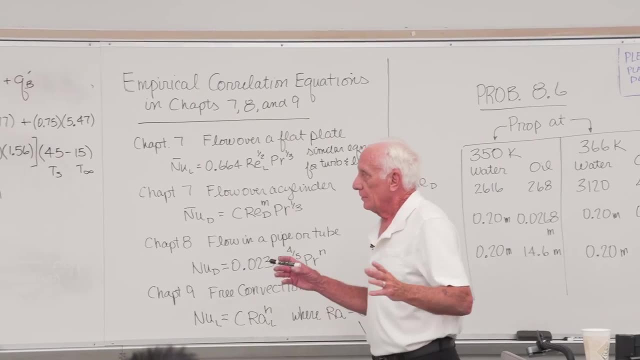 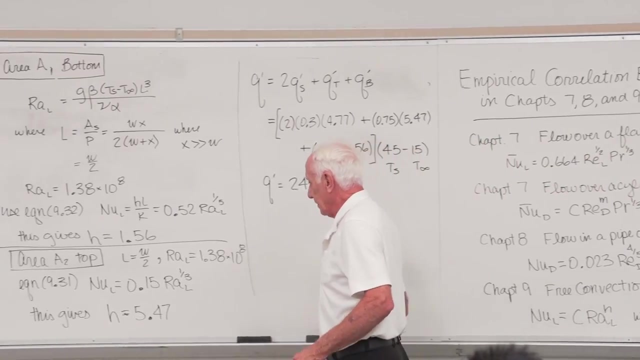 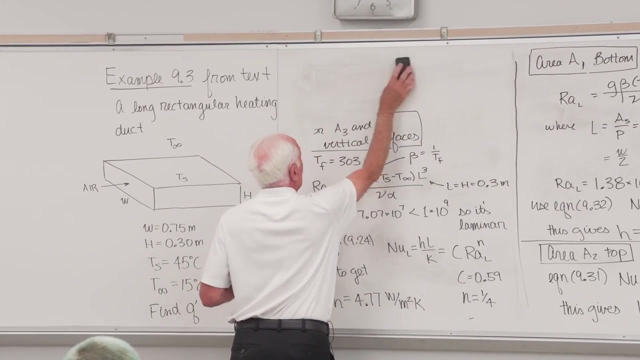 Any questions on that then? Okay, Now what's left? Horizontal and vertical cylinders, Okay. So now we'll do a- let's make some room right here. Let's do a vertical cylinder. We'll do both of them, for example problems, but we'll do the vertical one first. 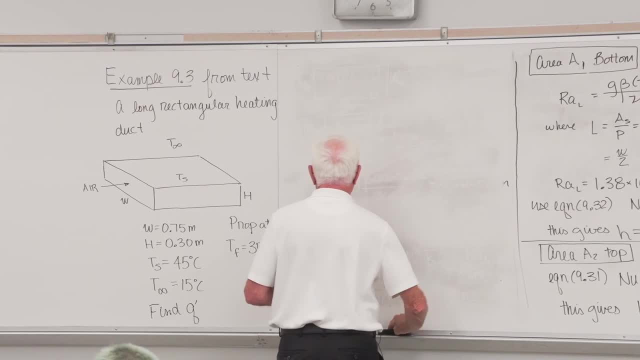 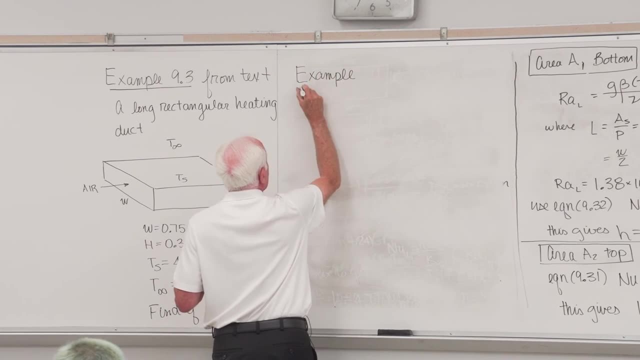 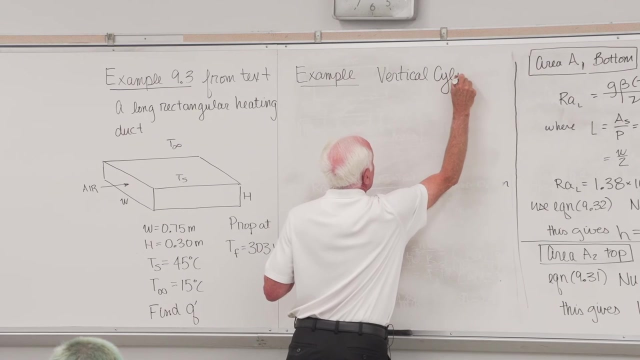 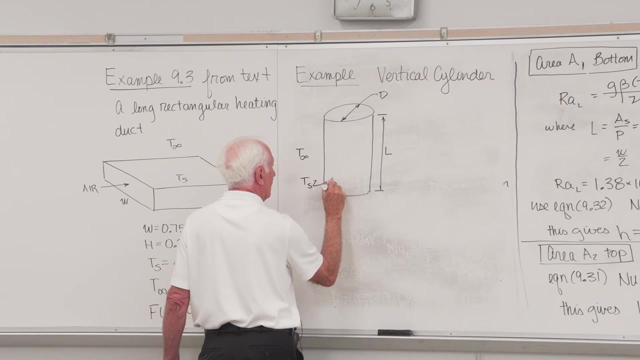 So example of vertical cylinder. Okay, So let's put some numbers in here: D: 20 centimeters diameter. L is one meter in height. T- infinity: 25 degrees. T surface is colder, 5 degrees Properties at T film. 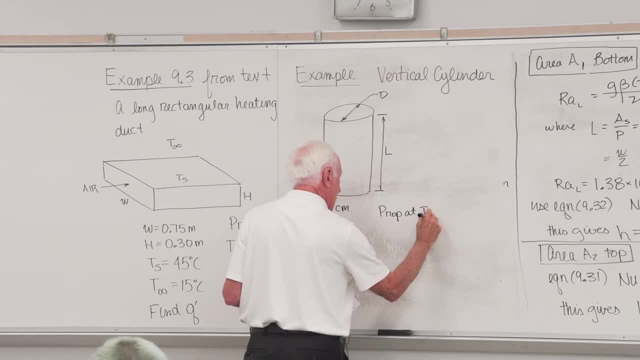 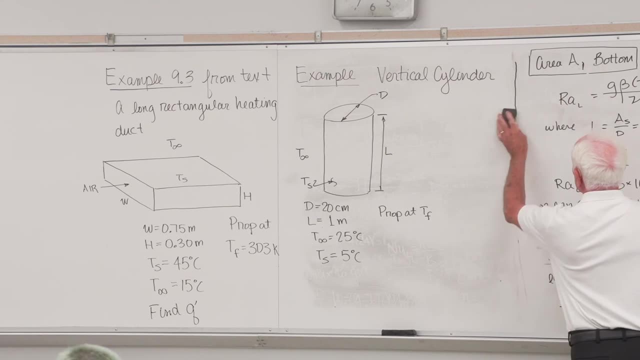 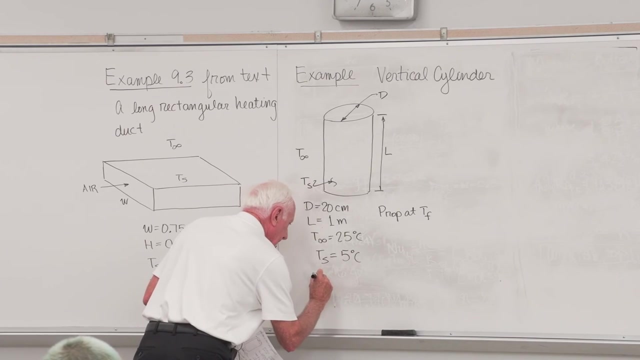 T surface is colder 5 degrees. Properties at T film: T surface is colder 5 degrees. Okay. So oh, and find Q. All right, we got everything we need. I think Property's at 288, T film is 288 Kelvin. 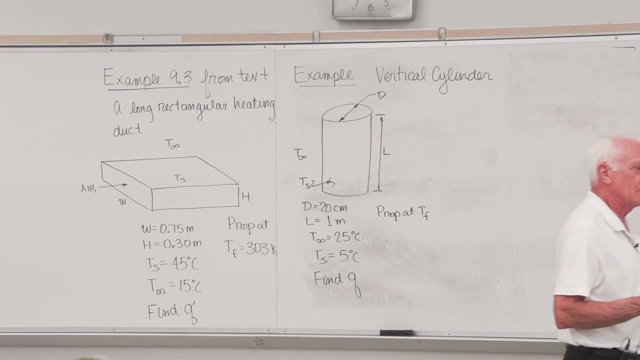 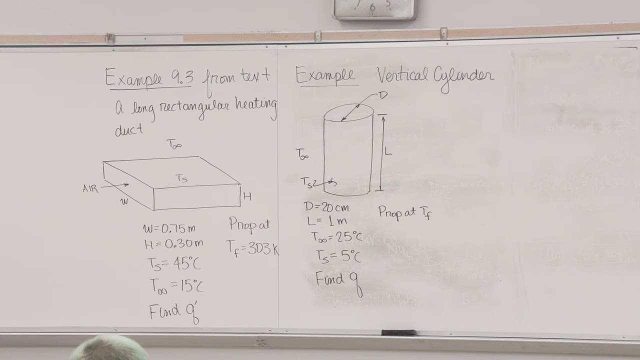 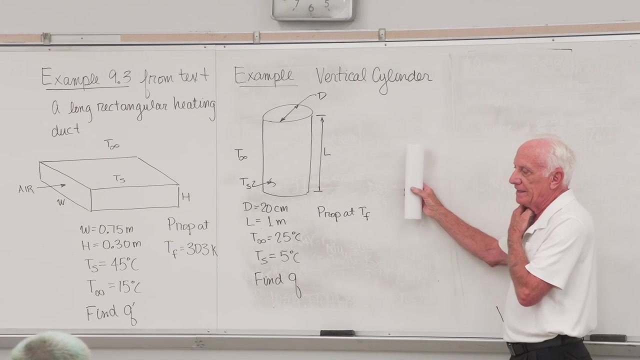 All right, we talked about it last time. We said: for a vertical cylinder, if you check a certain number and it satisfies an inequality, then you can model the vertical cylinder as if it is a vertical plate. We talked about that last time. 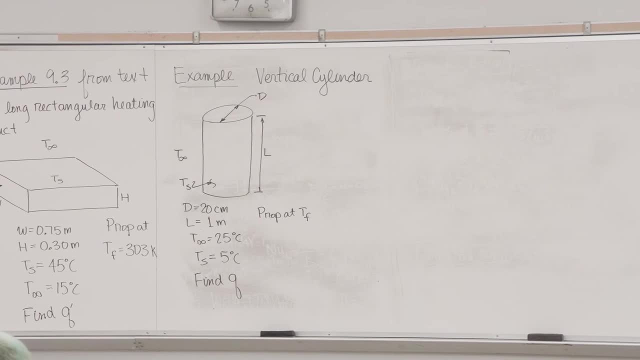 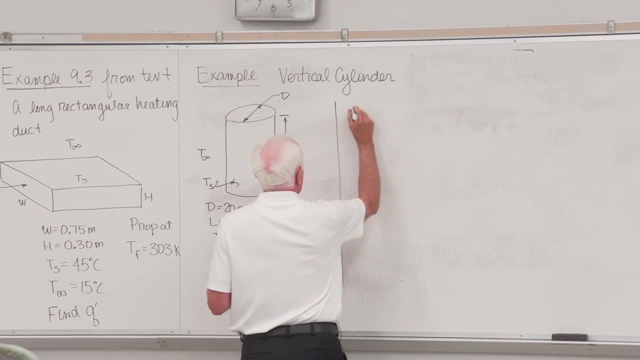 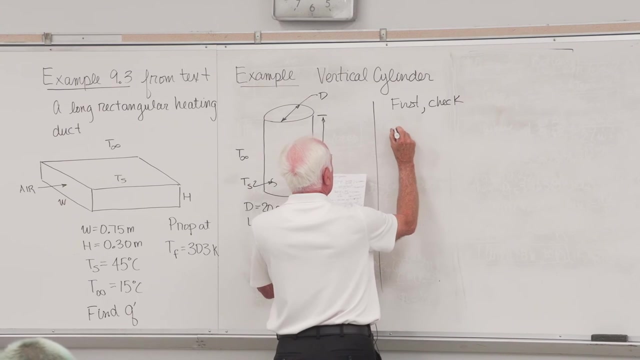 But you've got to check to see if that can be true. So we have to check this First. check D over L greater than or equal, I don't know yet- 35 over the Grashof number to the one-fourth. 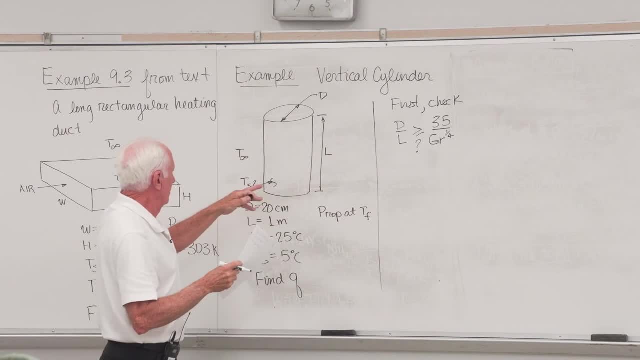 If that's true, I can use the equations for a vertical surface to solve this problem. Grashof, chapter nine: dimensionless parameters: Nussel, Rayleigh, Grashof, Prandtl- four of them. Okay, we haven't done Grashof yet. 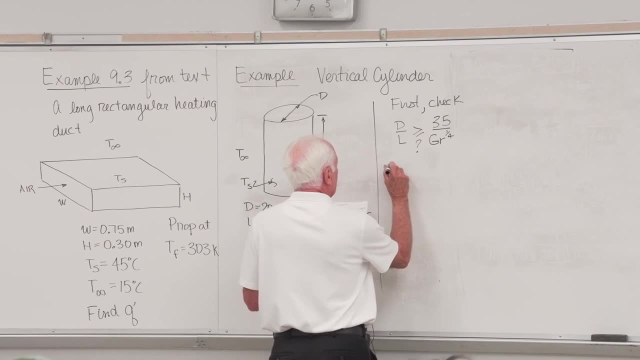 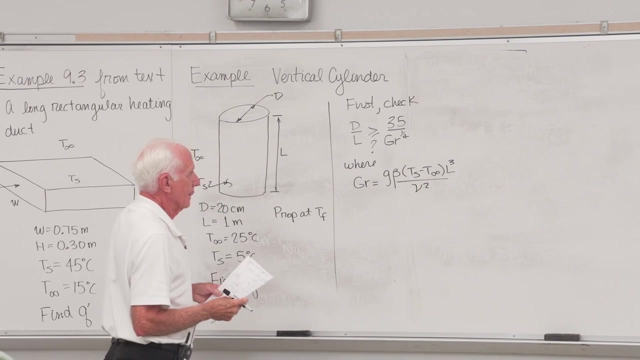 Okay, Grashof number Where Grashof G, it looks like Rayleigh almost. it's a little different. T S minus T, infinity L cubed divided by nu, squared Here. it is right here, Grashof. 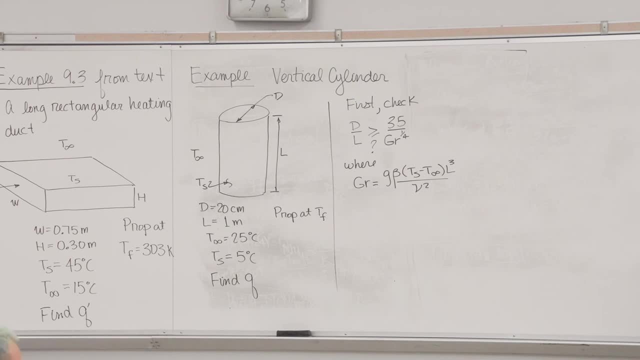 Grashof, Rayleigh over Prandtl. Okay, so we know everything. G 9.81,, beta 1 over T film absolute. We know T S, we know T infinity. Always put the hot temperature there first. 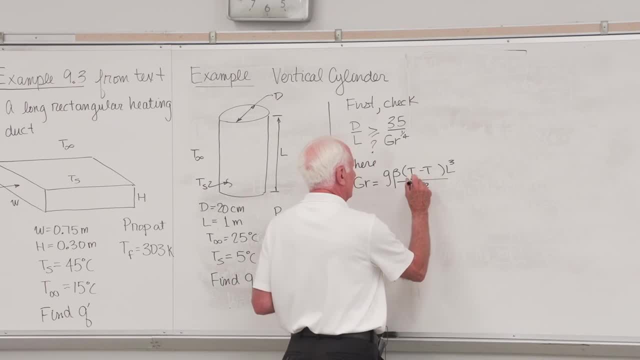 You don't want a negative Grashof number: T infinity minus T surface. Okay, Oh, I'm sorry, It is the opposite way. The T surface is 45,. excuse me, Oops, I'm not going the wrong way. 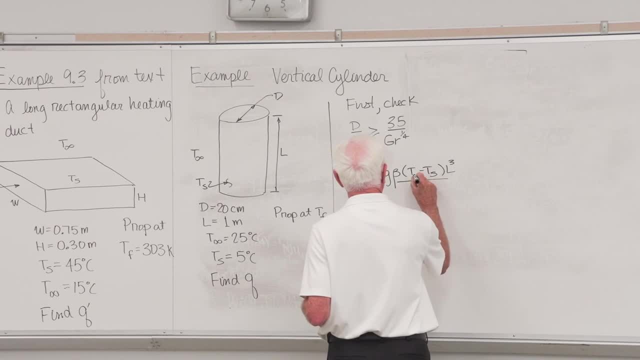 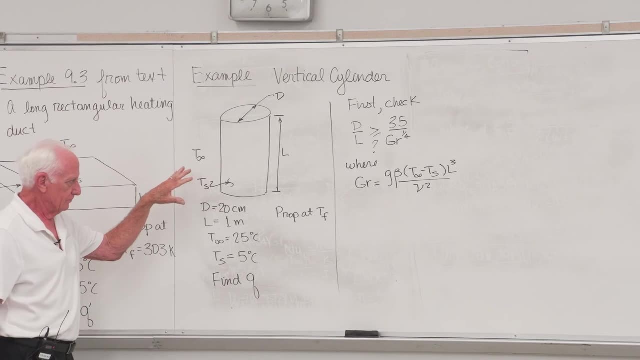 It is: Get rid of that guy. So we have T infinity, T infinity 25, T- surface. Now that's a good point, because what's happening here? That cylinder is cold, The air is warm, There's going to be a boundary layer and it starts up here. 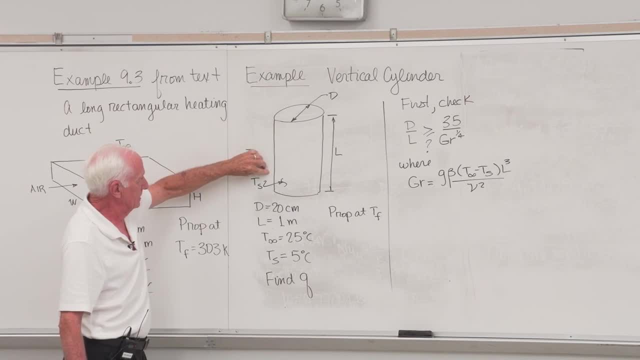 That's X equals zero, And it gets bigger as it goes down this way. That's X equals L. Okay, Again in chapter 9, there's either two symbols: in the Nusselt and the Grashof and in the Rayleigh. 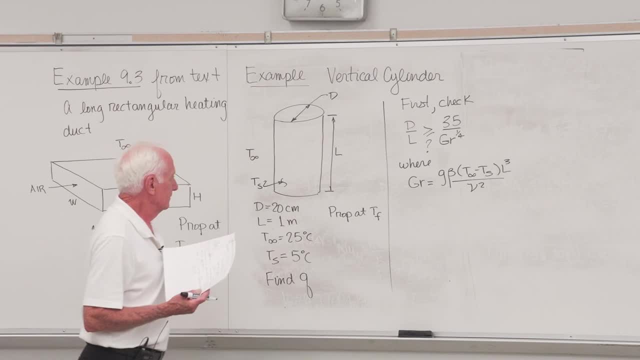 It's either an L or a D. Normally we would use D for this, but we're going to check just to see if we can approximate it by a plane surface where this is L, So we show that as L in here, Okay. 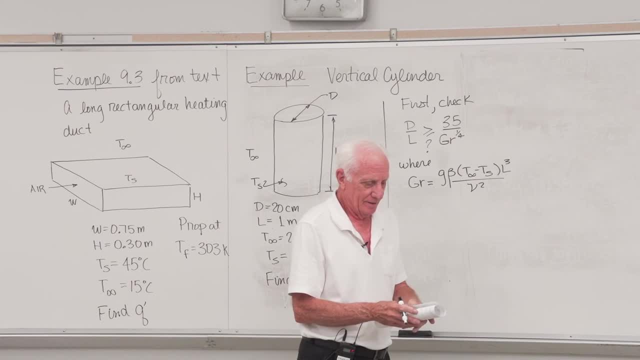 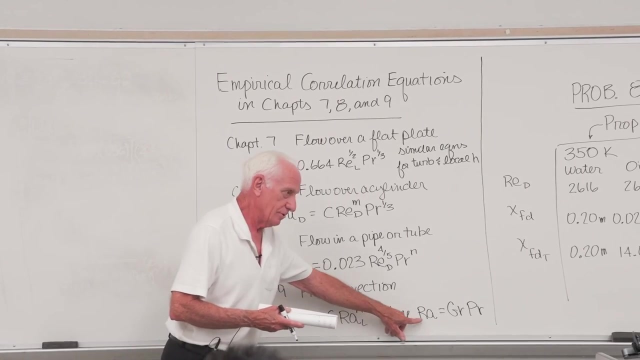 When we get to horizontal surfaces, horizontal pipes. guess what we use now? Oh, we use diameter. now It's a diameter. It's a diameter in there. It's a diameter in there. It's a diameter in there If it's horizontal diameter. 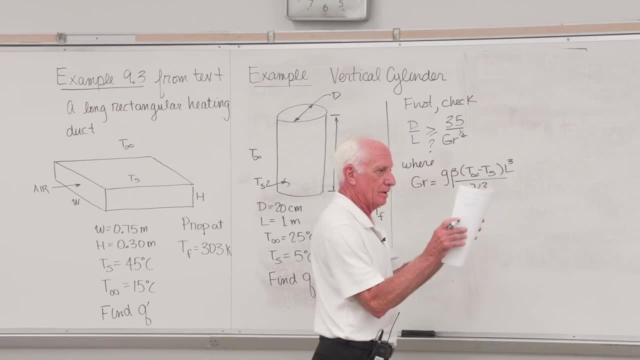 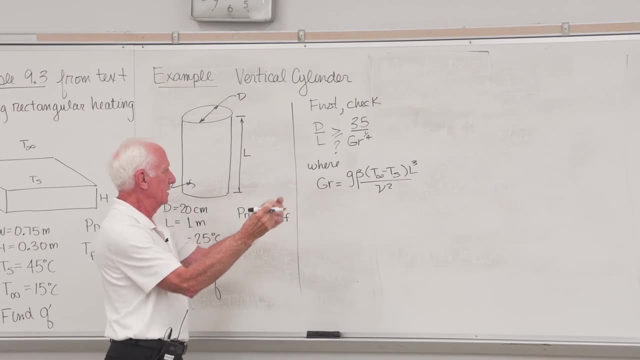 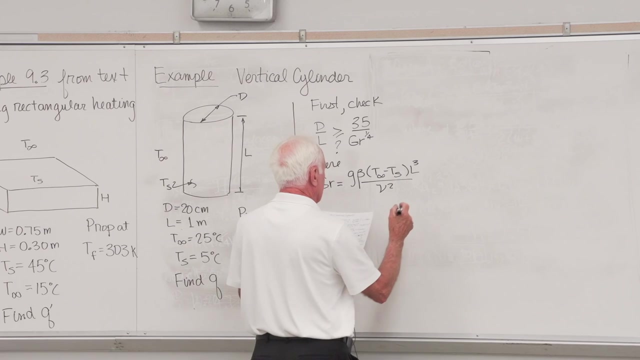 If it's vertical- and this is true- we use the height, Expand the cylinder out flat. Now it's a flat plate. Okay, So go ahead there and get that guy. then Grashof is equal to 3.085 times 10 to the ninth. 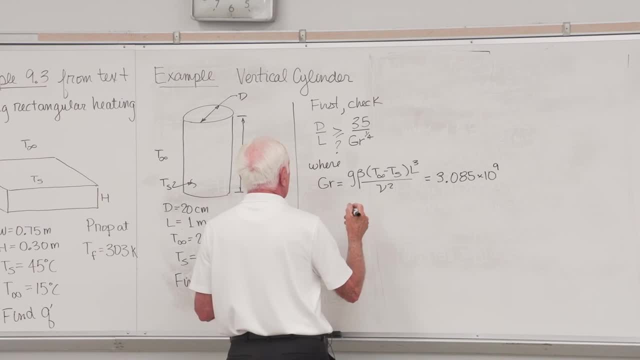 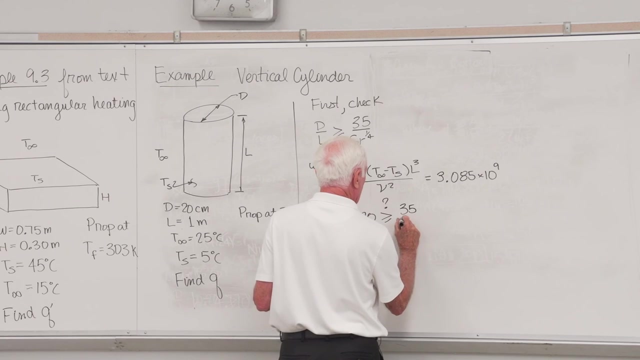 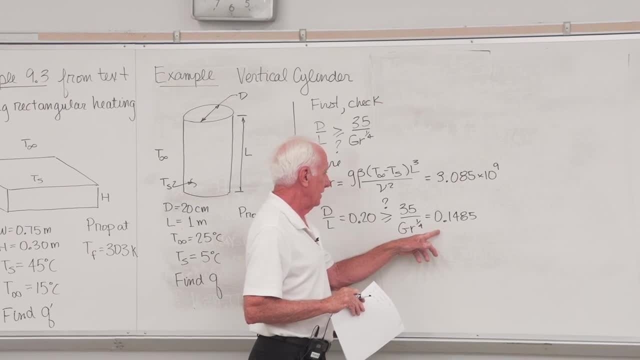 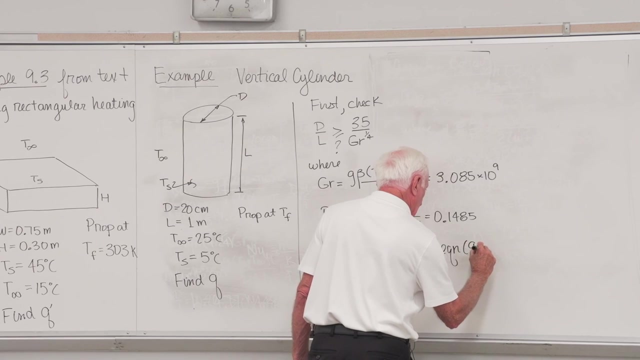 0.1485.. 0.1485.. 0.1485.. 0.1485.. 0.2 greater than 0.1485,. yes, can use equation 924.. Nusselt based on L. 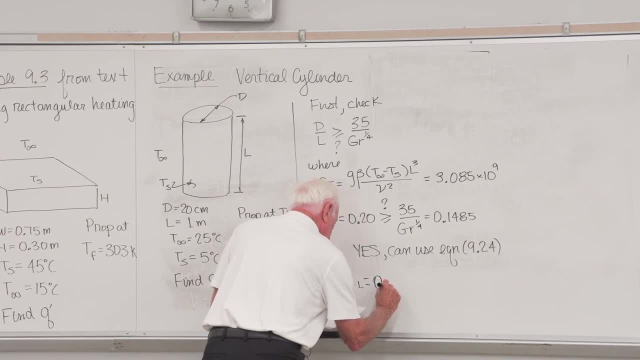 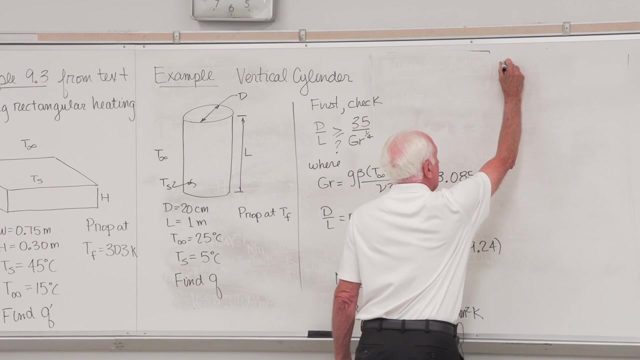 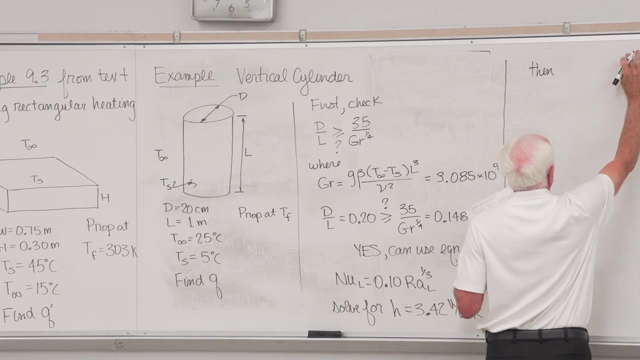 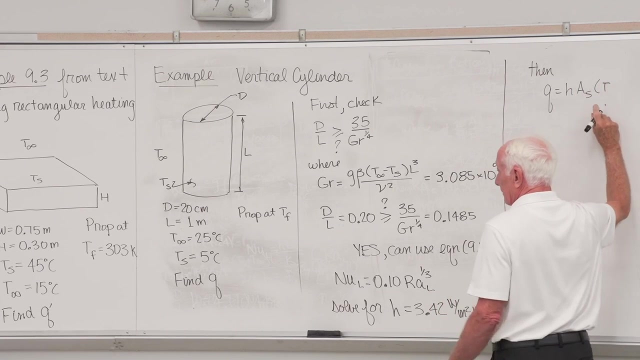 0.10, really L to the one-third. That's the equation solved for H, 3. 0.42.. 0.42.. Then Q equal H. A surface T: what's hot infinity. 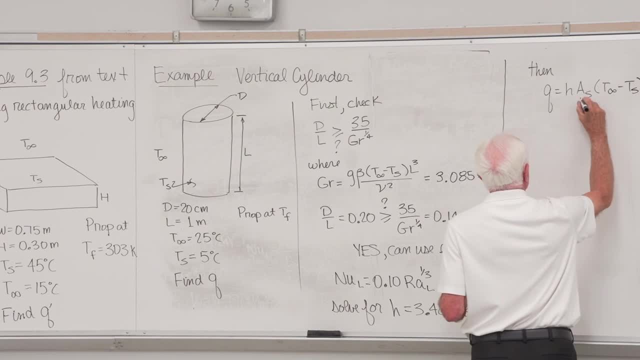 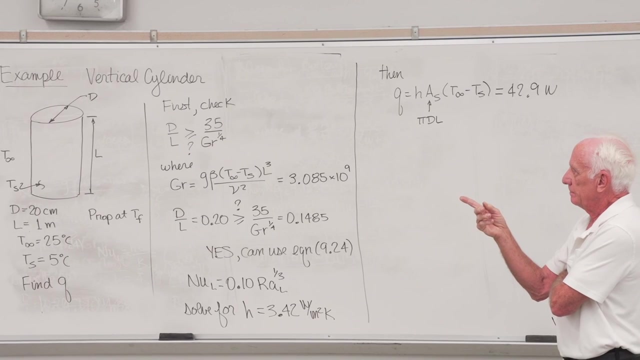 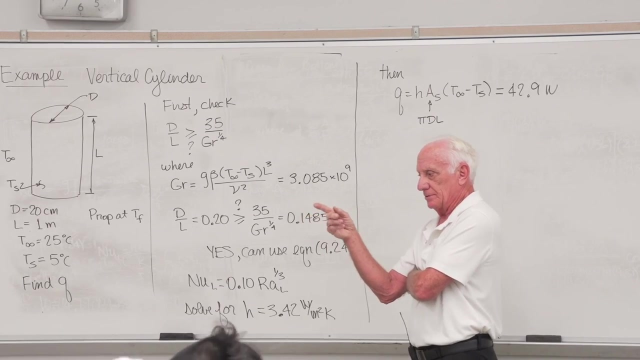 minus T surface Surface Surface Pi D L- 42.9 watts. 42.9 watts. So this is the fourth of the five geometries. Vertical surface: Vertical cylinder. Horizontal surface- hot. Horizontal surface cold.